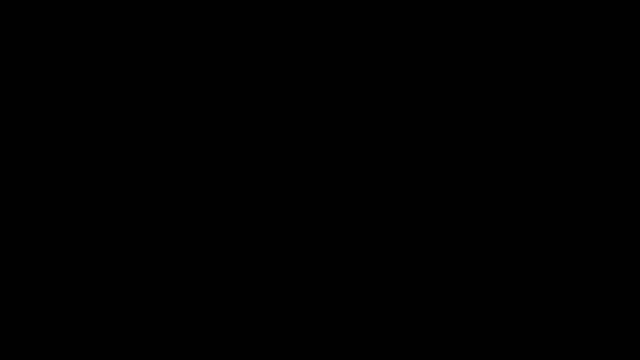 In this video we're going to focus on solving absolute value equations. Now I recommend that you watch this video to the end, because the problems they're going to start off easy, but over time they're going to get harder and harder. So stay tuned. Let's start with some 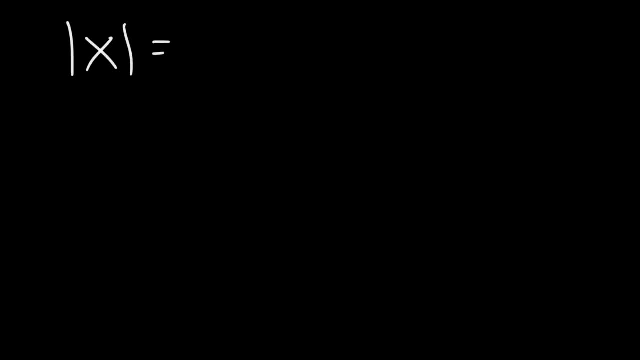 basics. Let's say, if we have the absolute value of x and it's equal to 9.. What is x equal to? What would you say Now? of course, x is equal to 9, but also you need to be aware that x can be. 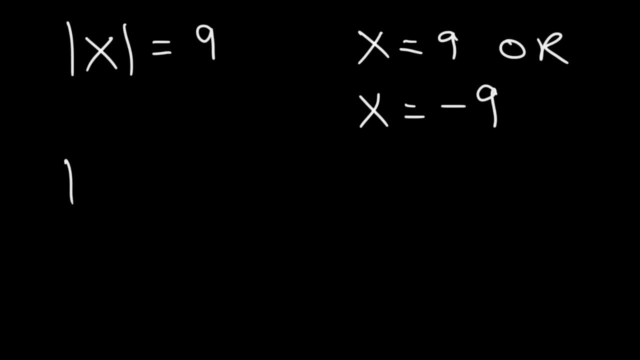 equal to negative 9.. Why do we say that The absolute value of 9 is 9, but also the absolute value of any negative number is equal to a positive number. So x can be 9 or negative 9.. So whenever you're solving an absolute value equation, you're going to have to be aware that 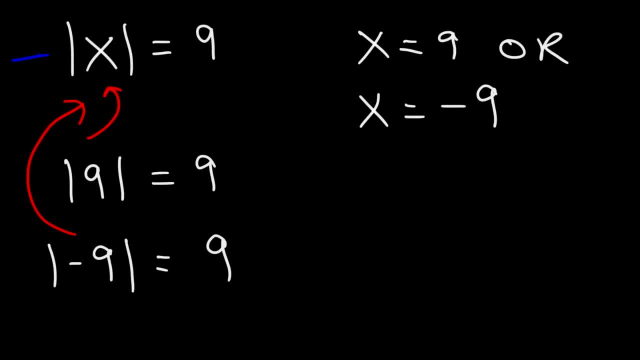 whenever you remove the absolute value, you need to put the positive answer or the answer the way it was, also the negative version as well. So whatever is on the right side, you can multiply it by negative 1 to get the second answer. So let's start with a simple example. 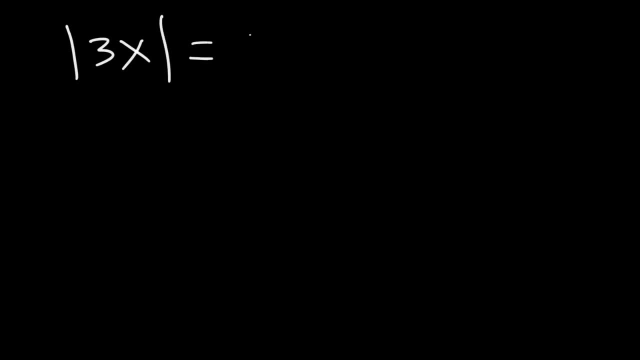 Let's say we have the absolute value of 3x is equal to 18.. What are the possible values of x? So we're going to write two equations: 3x is equal to 18.. And the second equation, 3x is equal to negative 18.. So if we divide both sides by 3,, 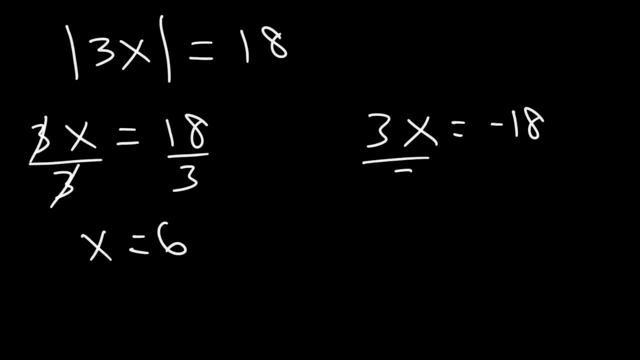 we're going to get, x is equal to 6.. On the other side, if we divide both sides by 3, x can be negative 6.. So we have two possible answers: 6 and negative 6.. Now here's another one. Let's say, if we have the absolute value of 5x plus 7 is 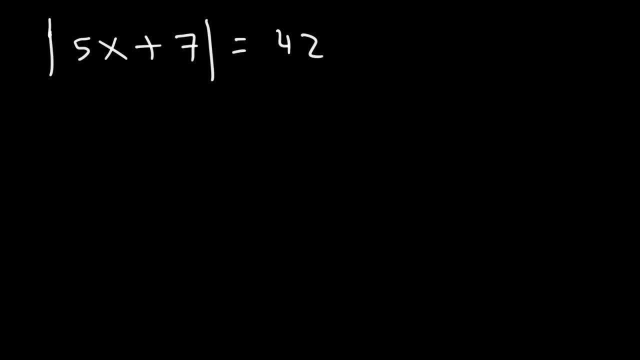 equal to 42. So go ahead and take a minute and try that example. So once again we're going to write two equations: 5x plus 7 is equal to 42. And 5x plus 7 is equal to negative 42.. 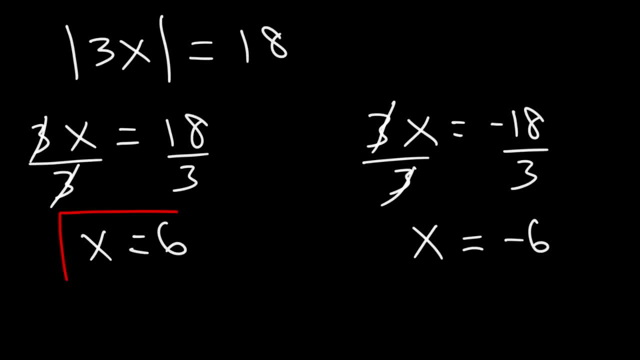 x can be negative 6.. So we have two possible answers: 6 and negative 6.. Now here's another one. Let's say, if we have the absolute value of 5x plus 7 is equal to 42. So go ahead and take a minute and try that example. So once again, we're going to write. 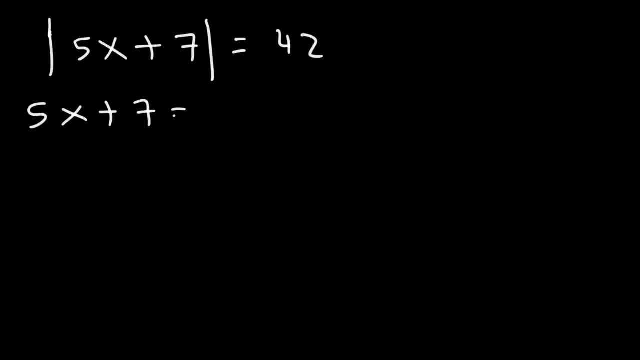 two equations: 5x plus 7 is equal to 42. And 5x plus 7 is equal to negative 42. So, working on the first one, we're going to subtract both sides by 7.. Now, 42 minus 7, that's 35.. Next we're going to divide both sides by 5.. And 35 divided by 5 is 7.. 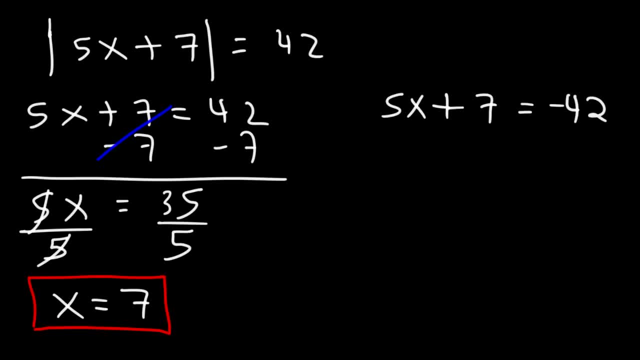 So this is the first answer. Now let's work on the second equation. Let's subtract both sides by 7. And so negative 42 minus 7 is negative 49. Now we could divide both sides by 5., And so we get a fraction as an answer: negative 49 over 5.. 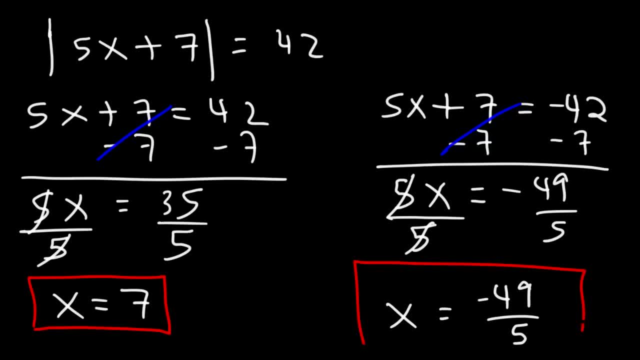 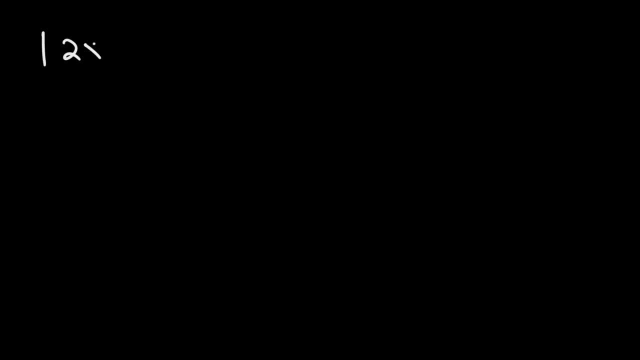 And that's the second answer. So that's how you can solve absolute value equations. Now let's work on another similar example. You can try this one for the sake of practice. Go ahead and calculate the value of x. So let's write two equations: 2x minus 3 is equal to 9.. 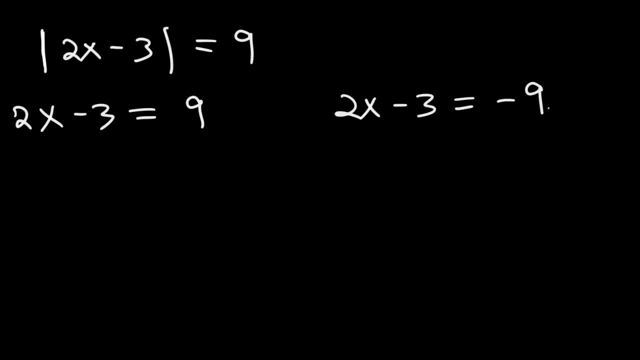 And 2x minus 3 is equal to negative 9.. So let's focus on the first one. 9 plus 3 is 12.. And then, if we divide both sides by 2, we're going to have 12 divided by 2.. 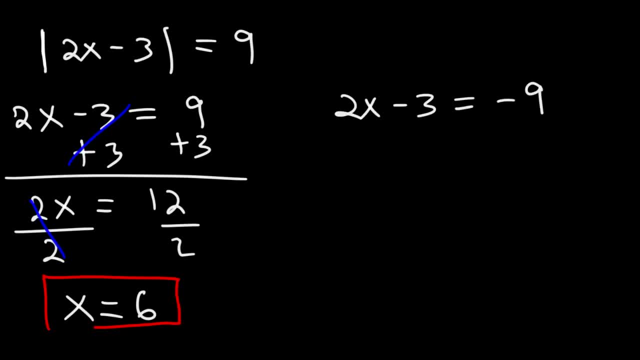 Which is 6.. And so this is the first solution. x is equal to 6.. Now for the second one: we're going to add 3 to both sides again, So this time we have negative 9 plus 3,, which is negative 6.. 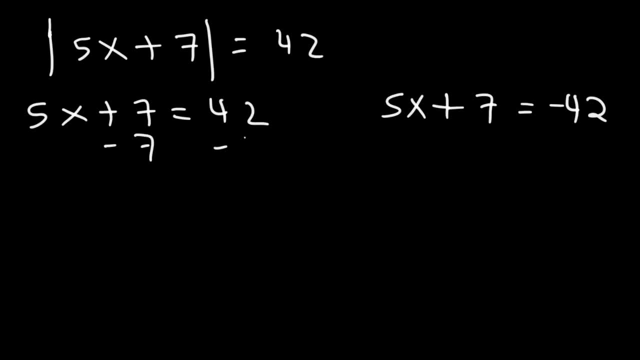 So, working on the first one, we're going to subtract x from 7.. We're going to subtract 6 from 7.. both sides by 7.. Now 42 minus 7, that's 35.. Next, we're going to divide both sides by. 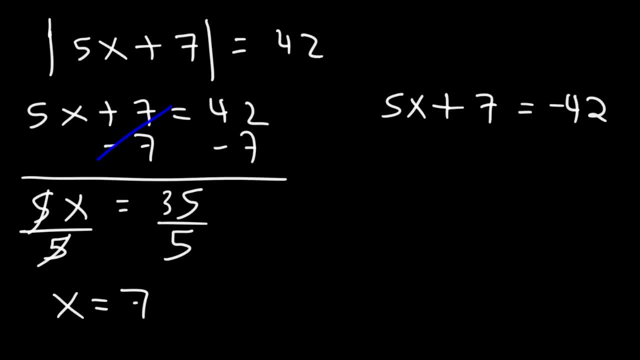 5. And 35 divided by 5 is 7.. So this is the first answer. Now let's work on the second equation. Let's subtract both sides by 7.. And so negative 42 minus 7 is negative 49.. 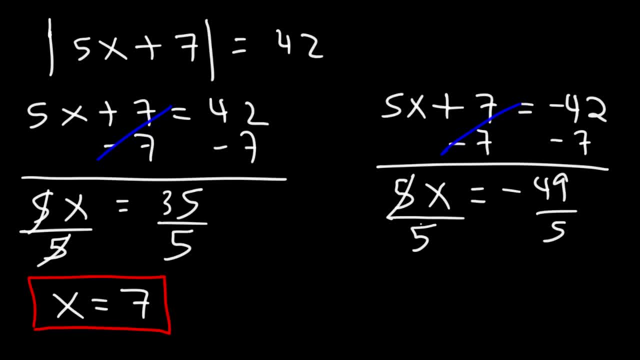 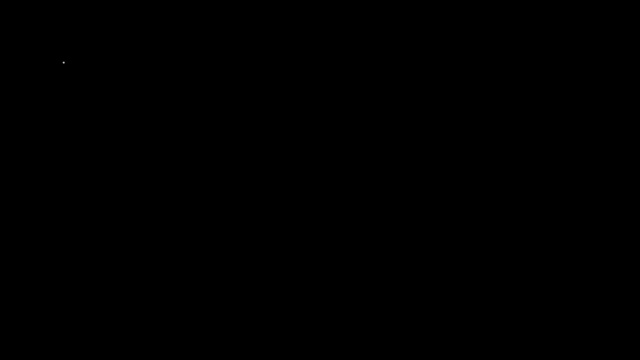 Now we could divide both sides by 5. And so we get a fraction as an answer: negative, 49 over 5.. And that's the second answer. So that's how you can solve absolute value equations. Now let's work on another similar equation. 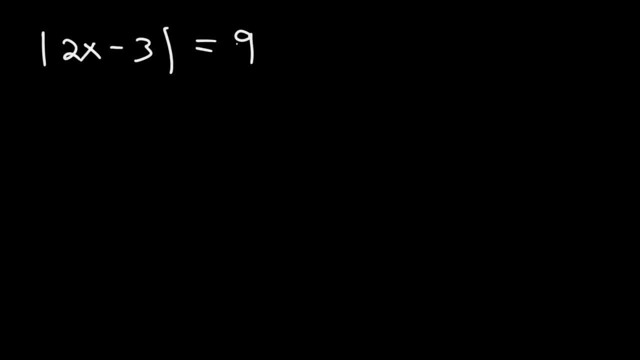 Another similar example. You can try this one for the sake of practice. Go ahead and calculate the value of x. So let's write two equations: 2x minus 3 is equal to 9.. And 2x minus 3 is equal to negative 9.. So let's focus on the first one: 9 plus 3 is 12.. And 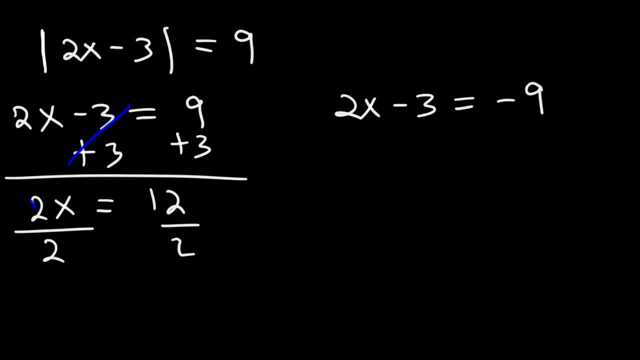 then if we divide both sides by 7,, that's 9.. And so we get a fraction as an answer. So let's divide both sides by 2.. We're going to have 12 divided by 2,, which is 6.. And so 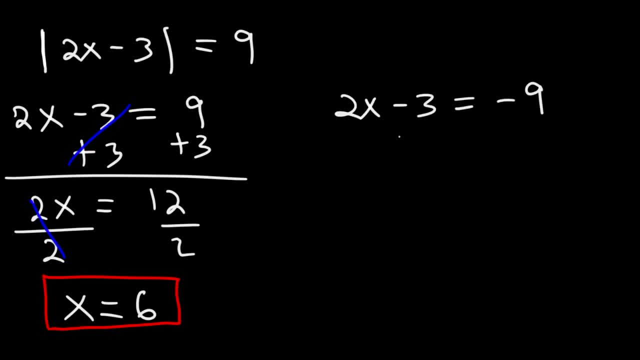 this is the first solution. x is equal to 6.. Now for the second one. we're going to add 3 to both sides again. So this time we have negative 9 plus 3, which is negative 6.. And then we're going to divide both sides by 2.. Negative 6 divided by 2 is negative. 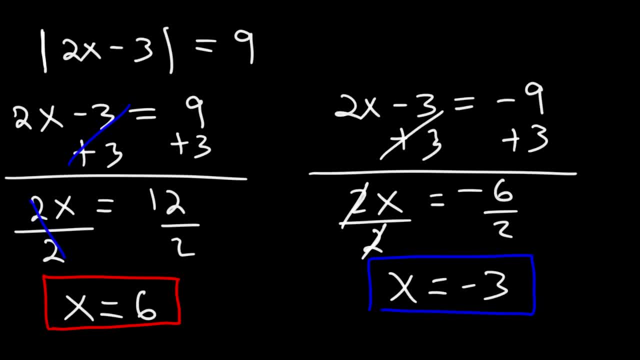 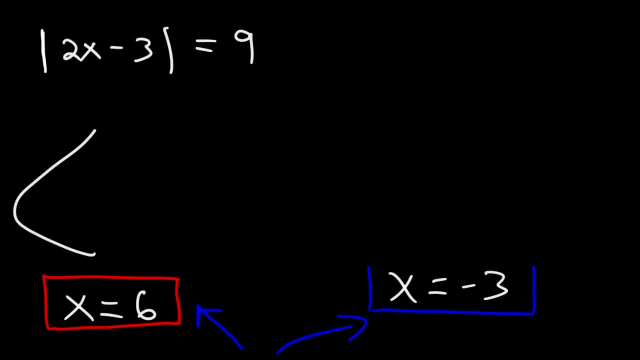 3.. So the two possible answers are positive 6 and negative 3.. So that's it for this example. Now, for those of you who want to check your work, here's what you can do: Take your x value and plug it in. So for the first one we're going to have, 2 times 6 minus 3 is equal. 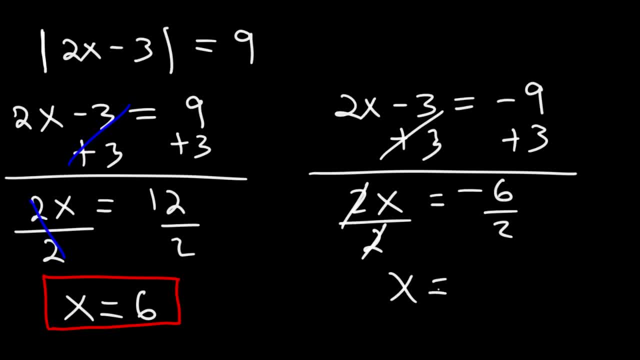 And then we're going to divide both sides by 2.. Negative 6 divided by 2 is negative 3.. So the two possible answers are positive 6 and negative 3.. So that's it for this one. Now, this example. 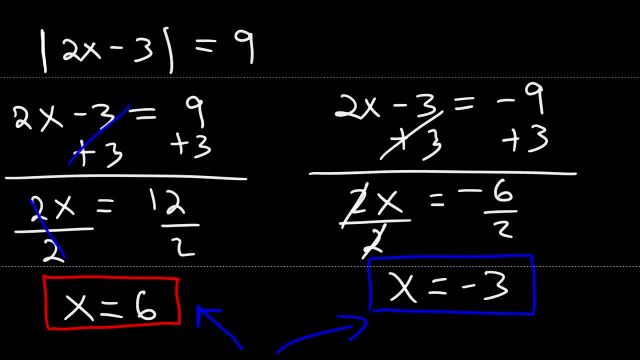 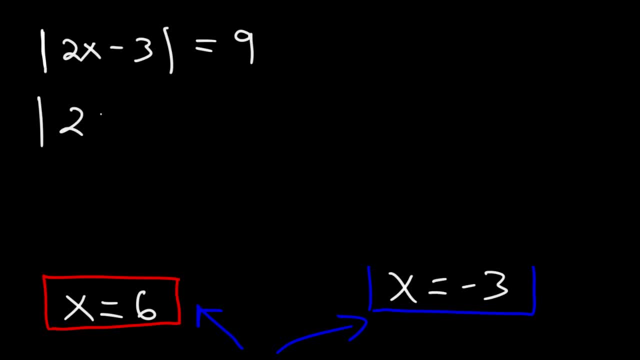 Now, for those of you who want to check your work, here's what you can do: Take your x value and plug it in. So for the first one we're going to have, 2 times 6 minus 3 is equal to 9.. 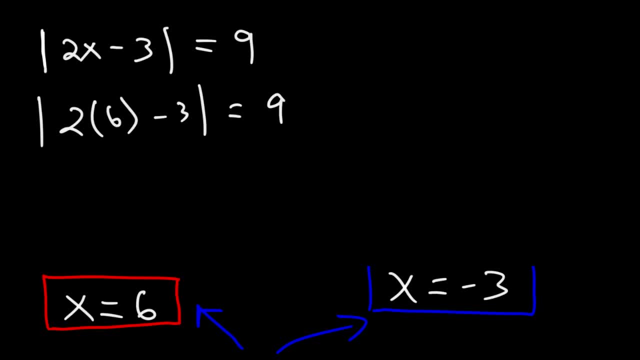 We're going to see if the value on the left side is equal to the value on the right side. 2 times 6 is 12. And 12 minus 3 is 9.. The absolute value of 9. Is 9.. 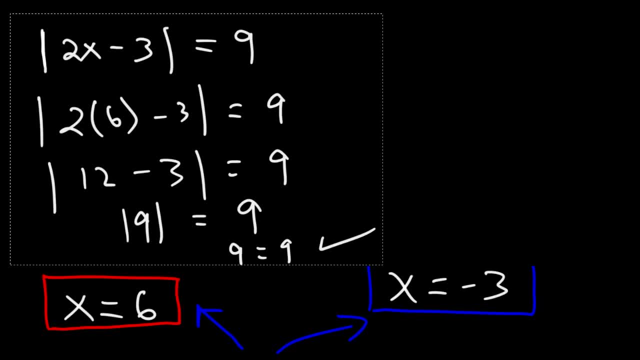 So the first solution works. Now let's try the second one to make sure it's correct. So let's replace x with negative 3.. 2 times negative 3 is negative 6.. And negative 6 minus 3 is negative 9.. 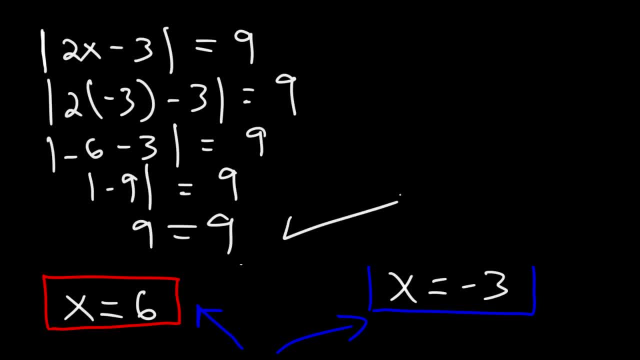 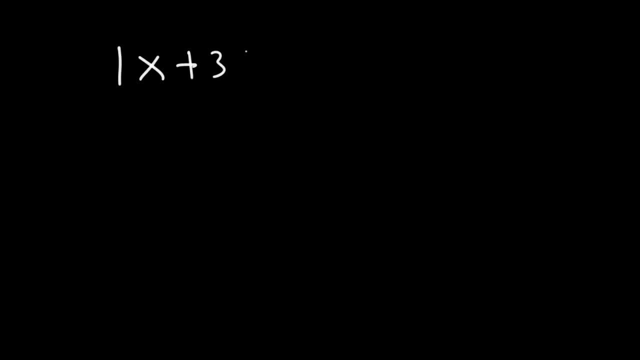 The absolute value of negative 9 is 9.. So this works as well. Now, what about this? Now, what about this one? The absolute value of x plus 3 is equal to negative 4.. Go ahead and try that Now. notice that there's no solution for this particular problem. 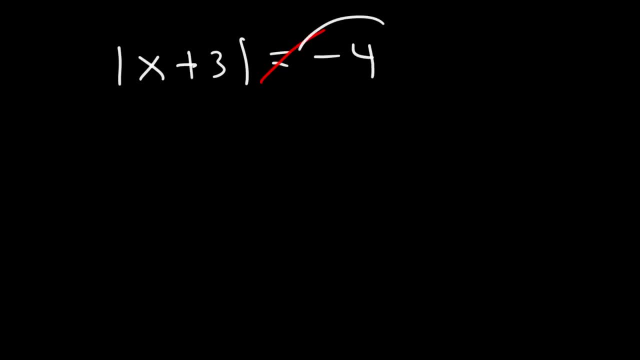 The absolute value of anything cannot equal a negative number. So anytime you see that if you see a negative on the other side- and on the left side there's nothing but an absolute value, then there's no solution. It doesn't matter what x value you decide to plug into this expression. 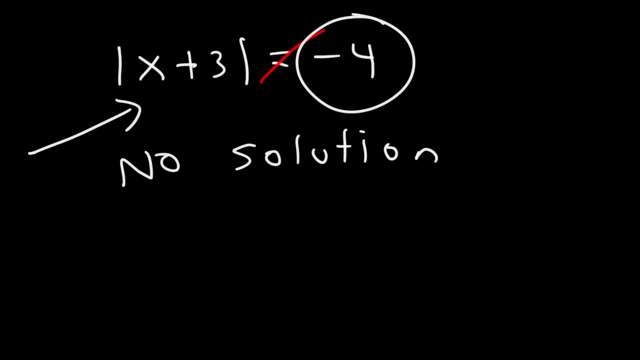 It's not going to give you a negative result. So watch out for questions like that. Now let's work on another one. Try that one. So once again, we're going to write two equations: 4x plus 6 over 5 is going to equal to positive 6, and it's going to equal negative 6.. 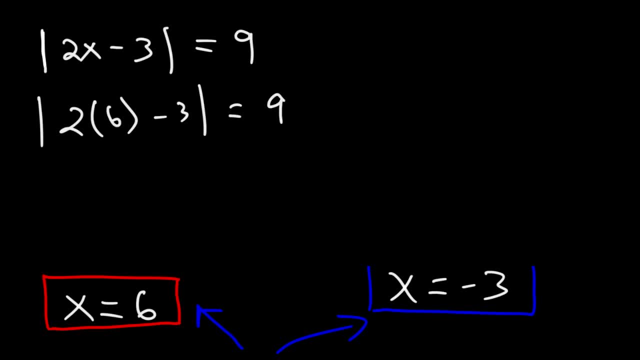 to 9.. We're going to see if the value on the left side is equal to the value on the right side, 2 times 6 is 12.. And 12 minus 3 is 9.. The absolute value of 9 is 9.. So the first solution. 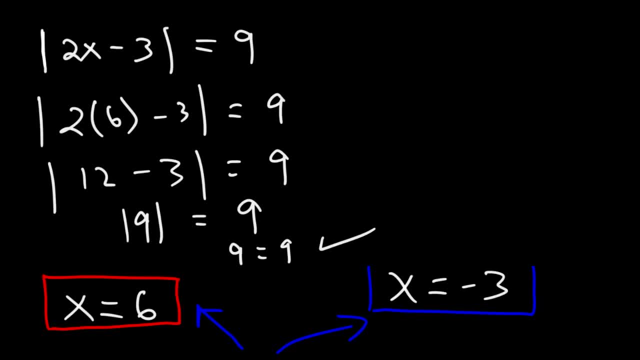 works. Now let's try the second one to make sure it's correct. So let's replace x with negative 3.. 2 times negative 3 is negative 6. And negative 6 minus 3 is negative 3.. 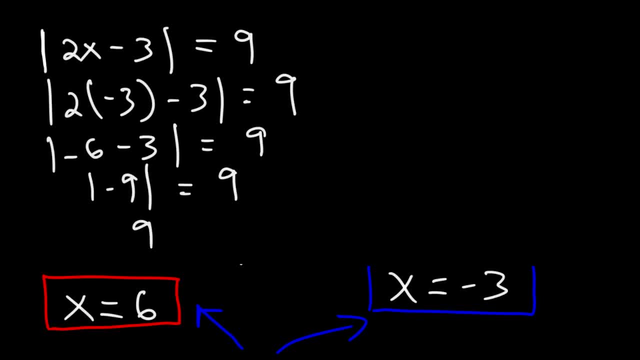 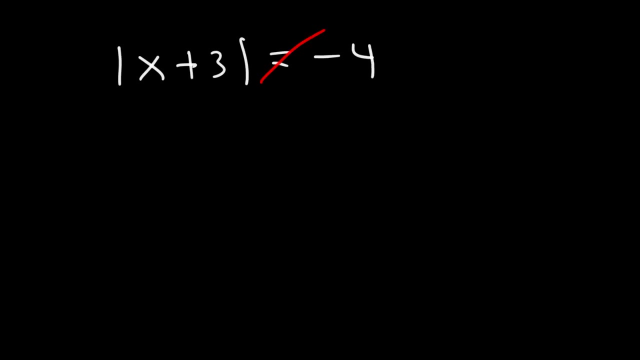 The absolute value of negative 9 is 9.. So this works as well. Now what about this one? The absolute value of x plus 3 is equal to negative 4.. Go ahead and try that Now. notice that there's no solution for this particular problem. The absolute value of 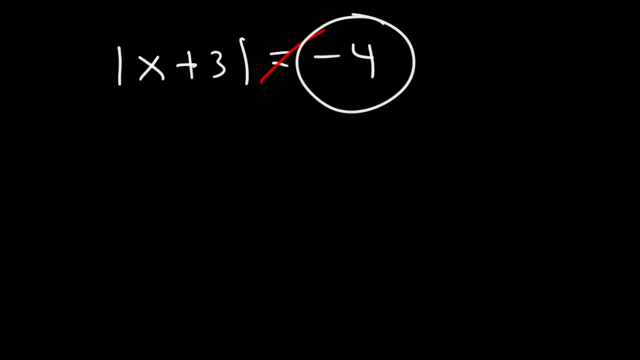 anything cannot equal a negative 4. So let's try that Nothing cannot equal a negative number. So anytime you see that if you see a negative on the other side and on the left side there's nothing but an absolute value, then there's. 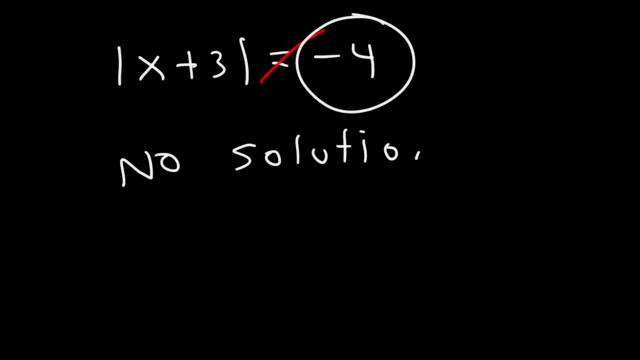 no solution. It doesn't matter what x value you decide to plug into this expression, It's not going to give you a negative result. So watch out for questions like that. Now let's work on another one. Try that one. So once again we're going to write two equations: 4x plus 6 over 5 is going to equal to positive 6, and it's going to equal negative 6.. 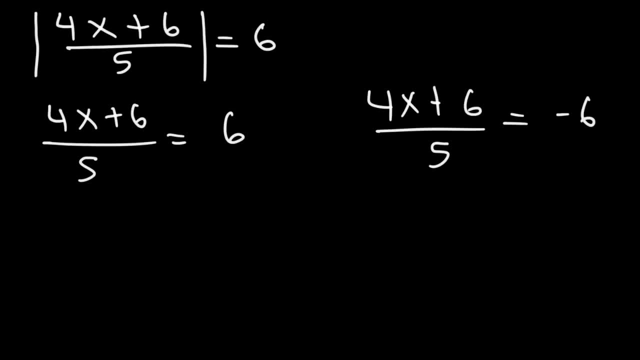 So let's start with the one on the left. What can we do to get rid of this fraction? What would you recommend? I recommend multiplying both sides by the denominator of that fraction. 5 divided by 5 is 1, so basically it cancels, leaving behind 4x plus 6 on the left side. Now, 6 times 5 is 30.. Next we need to subtract both sides by 6.. 30 minus 6 is 24, and then we need to divide both sides by 4.. So 24 divided by 4 is equal to 6.. So that's the first answer. 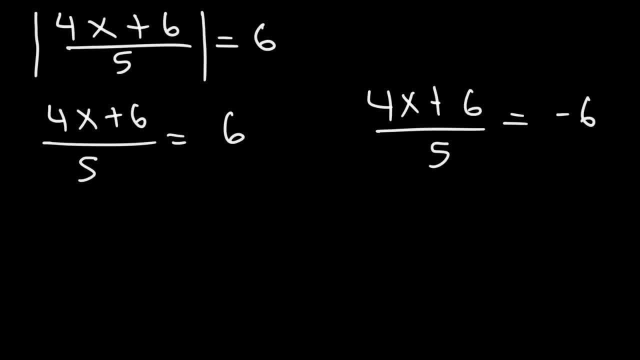 So let's start with the one on the left. What can we do to get rid of this fraction? What would you recommend? I recommend multiplying both sides by the denominator of that fraction. 5 divided by 5 is 1, so basically it cancels. 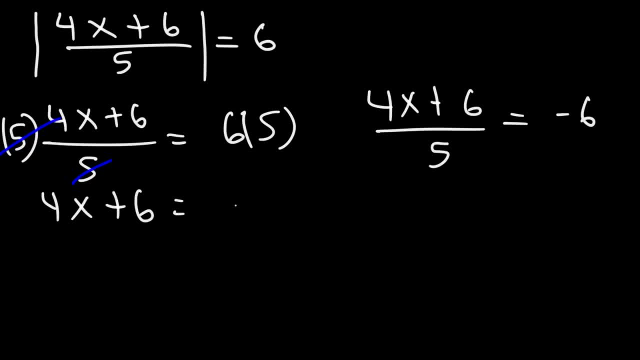 I'm leaving behind 4x plus 6 on the left side. I'm leaving behind 4x plus 6 on the right side. I'm leaving behind 4x plus 6 on the left side. I'm leaving behind 4x plus 6 on the right side. 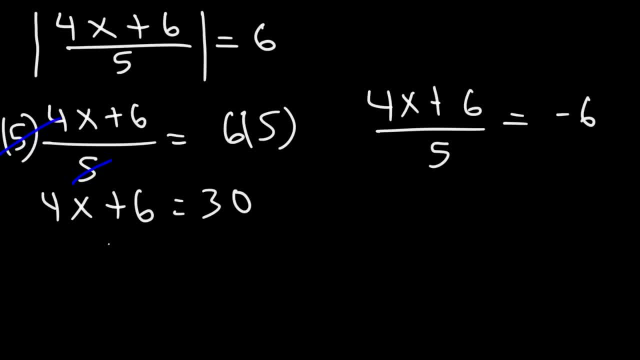 I'm leaving behind 4x plus 6 on the left side. Now, 6 times 5 is 30. Next we need to subtract both sides by 6.. 30 minus 6 is 24.. And then we need to divide both sides by 4.. 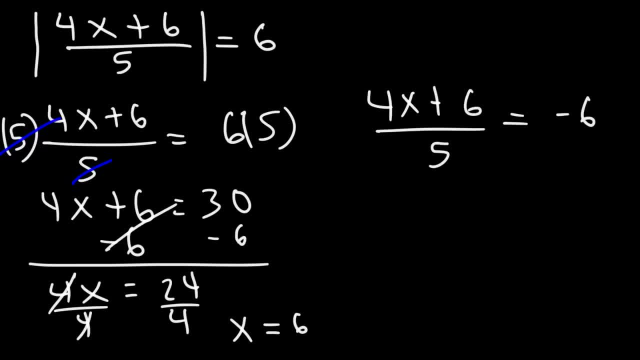 So 24 divided by 4 is equal to 6.. So that's the first answer. Now for the second one. we're going to do the same thing. We're going to multiply both sides by 5.. Okay, And so we're going to get: 4x plus 6 is equal to negative 30.. 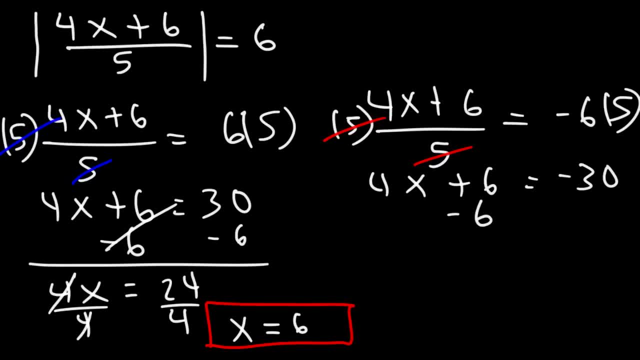 And then we're going to subtract by 6.. So negative 30 minus 6 is negative 36. And then we can divide both sides by 4.. Negative 36 divided by 4 is negative 9.. And so that is the second answer. 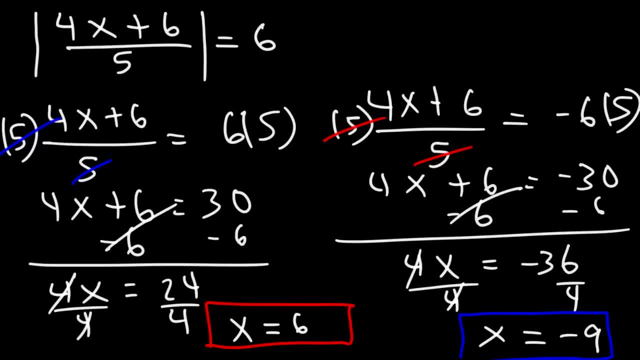 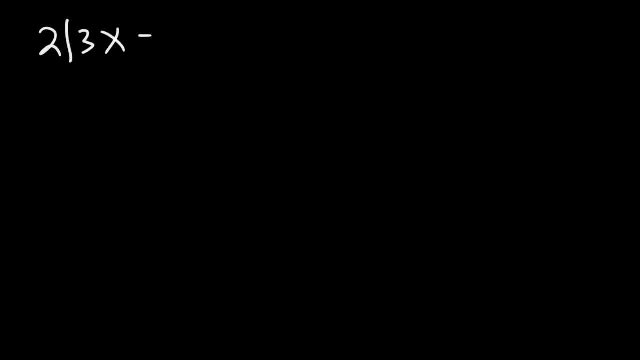 So x can equal positive 6. Or x can equal negative 9.. Now what if you were to get a problem that looks like this? What would you do in a situation like this? Now, here's what you should not do At this point: you should not write two equations. 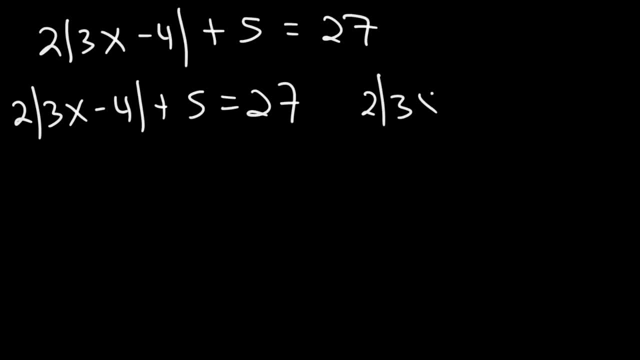 So you shouldn't make this 27.. And then write another equation. So you shouldn't make this 27.. Write another equation where this is equal to negative 27.. So why is that? Why should we not write two equations at this point? 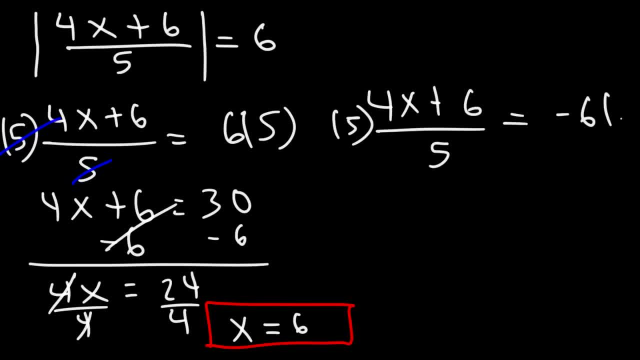 Now for the second one. we're going to do the same thing. We're going to multiply both sides by 5.. And so we're going to get: 4x plus 6 is equal to negative 30, and then we're going to subtract by 6.. So negative 30 minus 6 is negative 36, and then we can divide both sides by 4.. 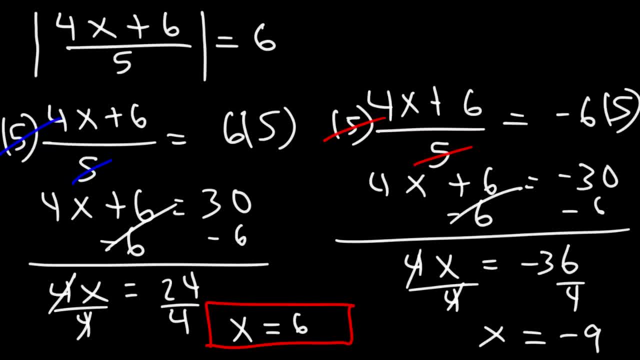 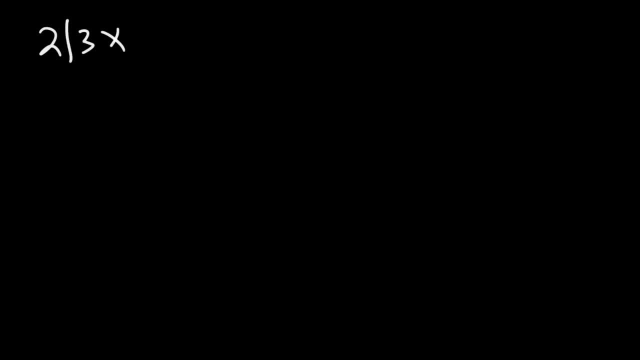 Negative 36 divided by 4. Is negative 9.. And so that is the second answer. So x can equal positive 6, or x can equal negative 9.. Now what if you were to get a problem that looks like this: 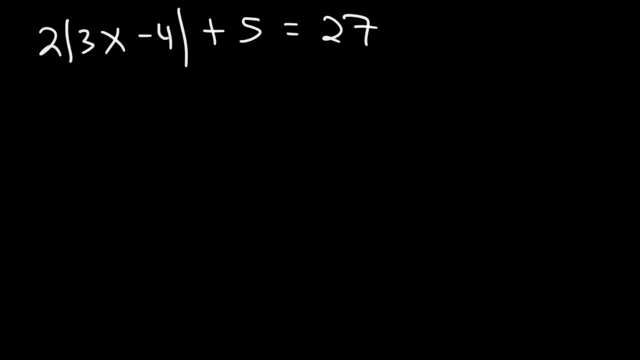 What would you do in a situation like this? Now, here's what you should not do At this point. you should not. You should not write two equations, So you shouldn't make this 27, and then write another equation where this is equal to negative 27.. 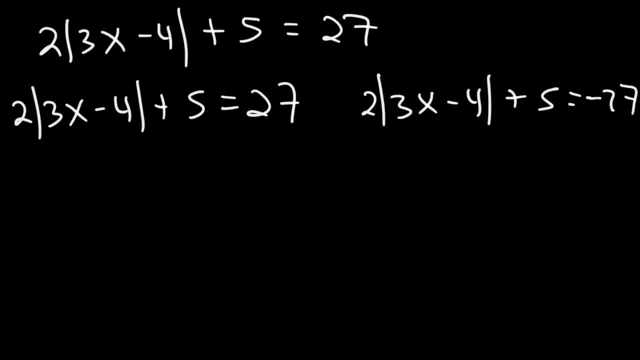 So why is that? Why should we not write two equations at this point? How do we know when we should write two equations and when we shouldn't Notice that we have numbers outside of the absolute value on the left side of the equation? 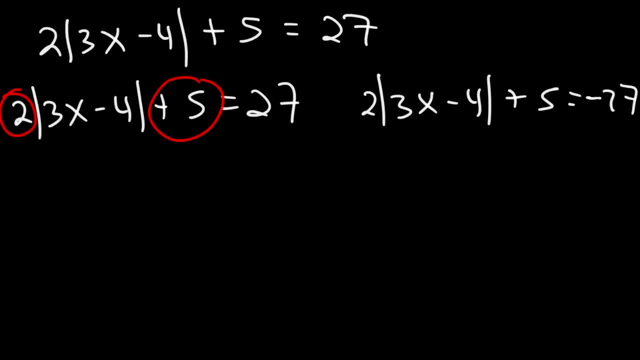 Whenever you see that You shouldn't break it up into two equations yet. You need to get rid of those numbers on the left side. Now, if I had, for example, 7x plus 3. I'm just going to make up something equal to 15.. 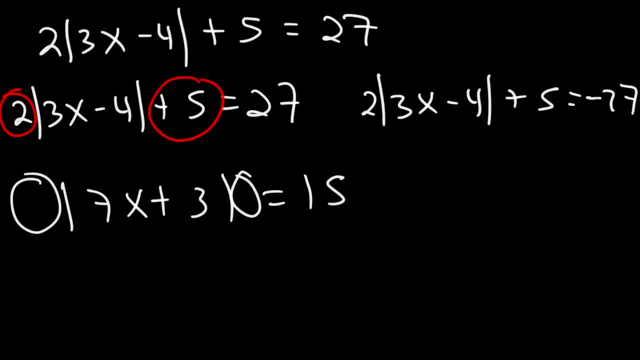 Notice that there's no numbers outside of the absolute value on the left side. So at this point I could break it up into two equations: 15 and negative 15.. But if I have numbers outside of the absolute value equation? 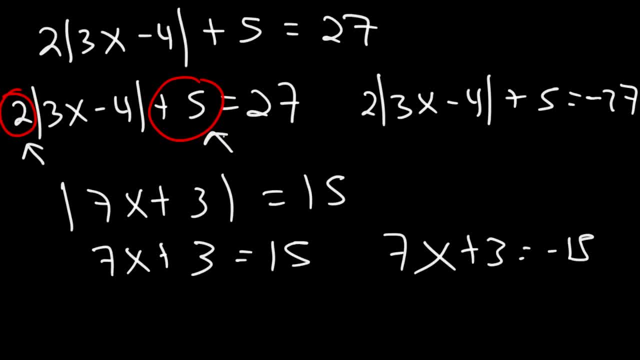 I need to simplify the equation first before breaking it up into two equations. So make sure you recognize that when you see it on a test. So the first thing we're going to do is subtract both sides by 5.. 27 minus 5 is 22.. 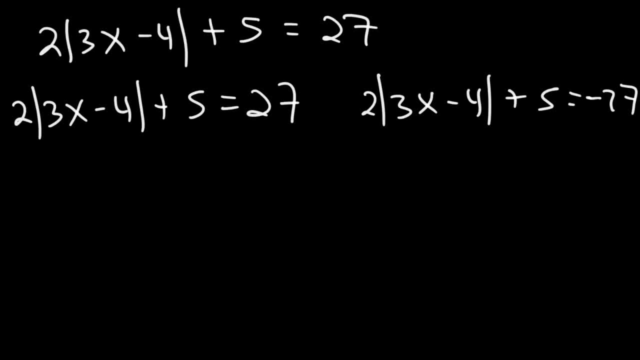 How do we know when we should write two equations and when we shouldn't Notice that we have numbers outside of the absolute value on the left side of the equation? Whenever you see that you shouldn't break it up into two equations yet, You need to get rid of those numbers on the left side. 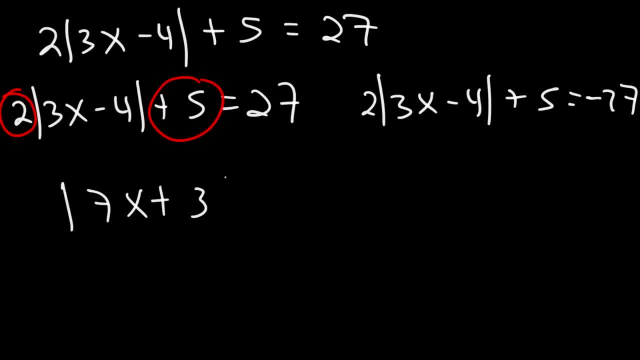 Now, if I had, for example, 7x plus 3, I'm just going to make up something equal to 15, notice that there's no numbers outside of the absolute value on the left side. So at this point I could break it up into two equations: 15 and negative 15.. 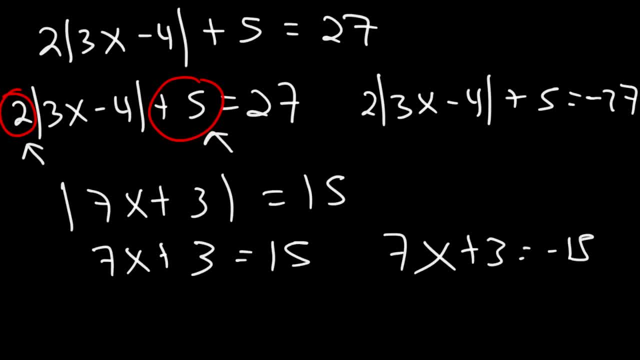 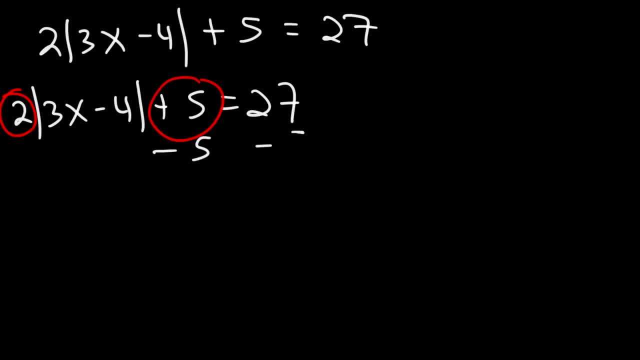 So the first thing we're going to do is subtract both sides by 5.. 27 minus 5 is 22.. And then we're going to divide both sides by 2.. And so now, at this point we have the absolute value of: 3x minus 4 is equal to 5.. 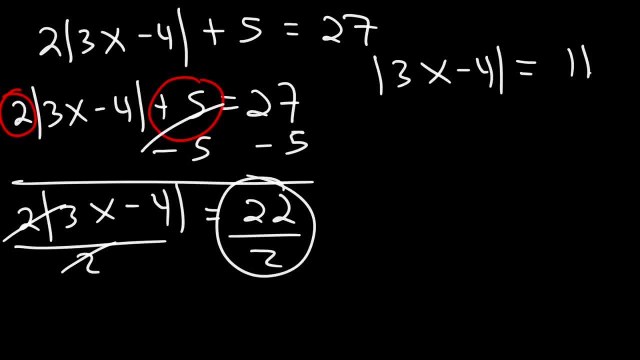 22 divided by 2, which is 11.. Now, at this point, notice that we have no numbers outside of the absolute value. So now we can break it up into two equations: 3x minus 4 is equal to 11.. 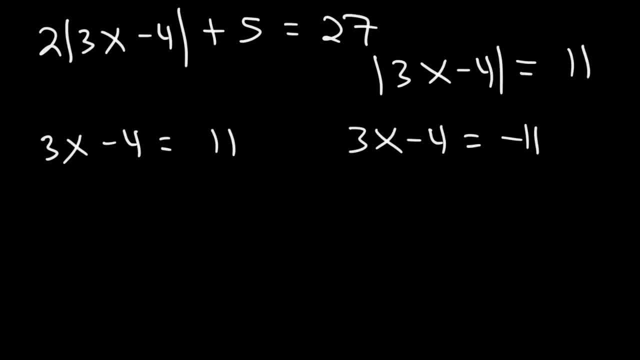 And 3x minus 4 is equal to negative 11.. So let's go ahead and solve it. 11 plus 4 is It should be zero. Now, if you have any other number out there, you should just go in here. 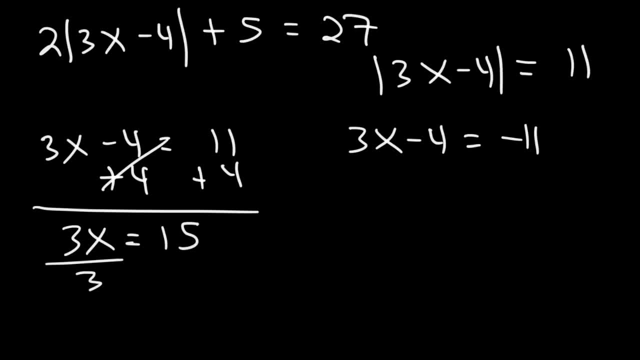 Go ahead is 15.. And 15 divided by 3 is 5.. Thus x is equal to 5.. That's the first one Negative. 11 plus 4 is negative 7.. And then, once we divide both sides by 3,, 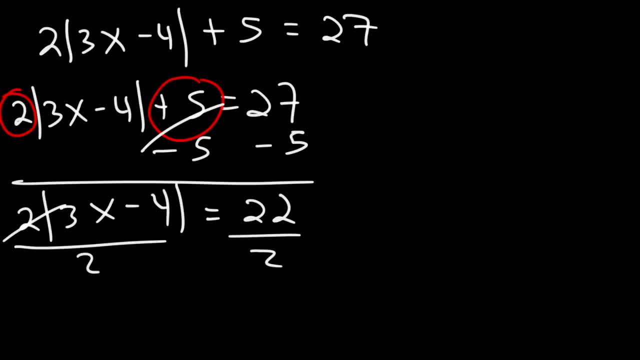 And then we're going to divide both sides by 2.. And so now, at this point, we have the absolute value of: 3x minus 4 is equal to 22 divided by 2, which is 11.. Now, at this point, notice that we have no numbers outside of the absolute value- 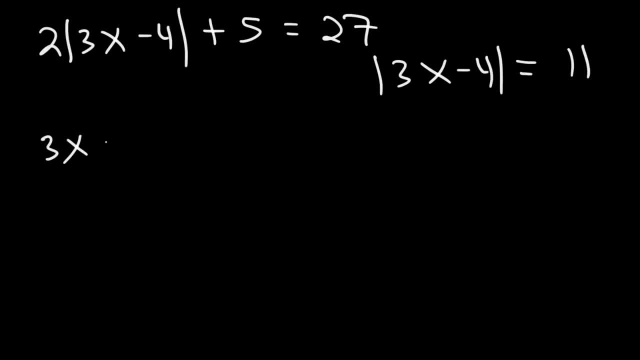 So now we can break it up into two equations: 3x minus 4 is equal to 11. And 3x minus 4 is equal to negative 11. So let's go ahead and solve it: 11 plus 4 is 15.. 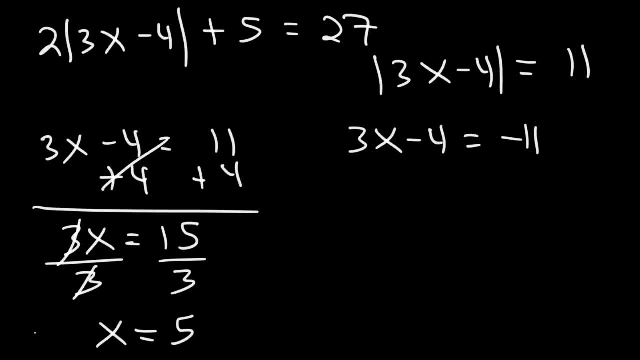 And 15 divided by 3 is 5.. Thus x is equal to 5.. That's the first one. Negative 11 plus 4 is negative 7.. And then, once we divide both sides by 3, the second answer will be equal to. 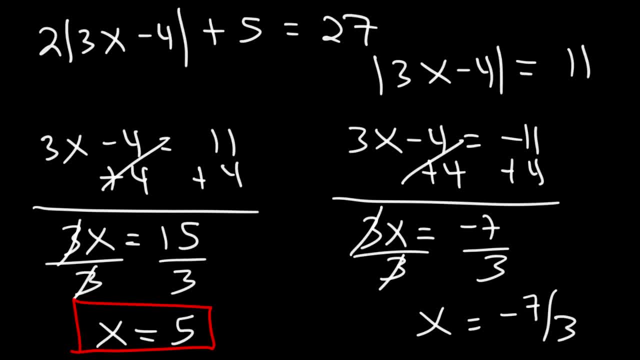 a fraction. So it's going to be negative 7 over 3.. So these are the solutions to the original equation And you can plug it in to see if it makes sense. if it works Now, let's go ahead and work on another example. 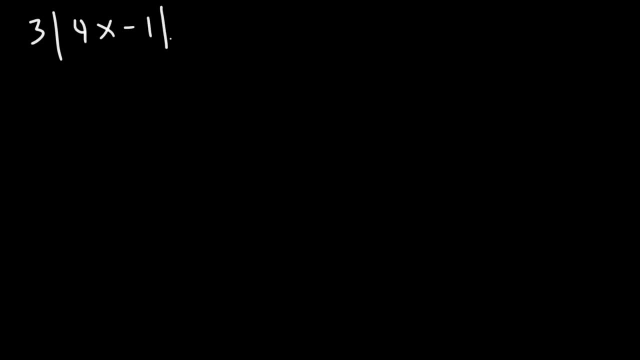 So we're going to have 3 times the absolute value of 4x minus 1 minus 5, which is equal to 16.. So for the sake of practice, let's pause the video and try that example. So we're going to begin by adding 5 to both sides of the equation. 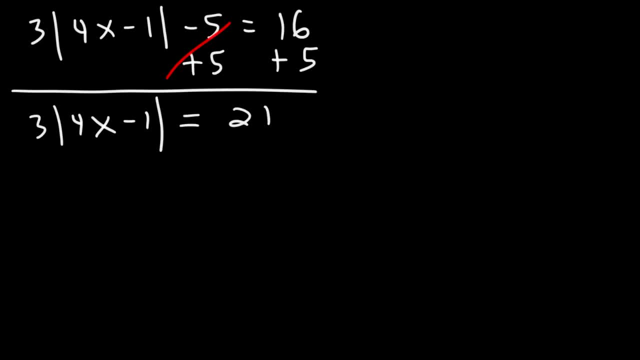 Now 16 plus 5 is 21.. Next, let's divide both sides by 3.. And so 21 divided by 3 is 7.. Now, in this case, we're going to have 3 times the absolute value of 4x minus 7.. 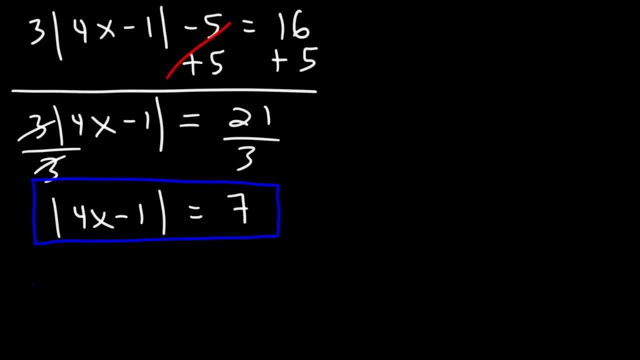 In this format. in this form, we can now break it up into two equations. So the first one is going to be: 4x minus 1 is equal to 7.. And the second one, 4x minus 1, is equal to negative 7.. 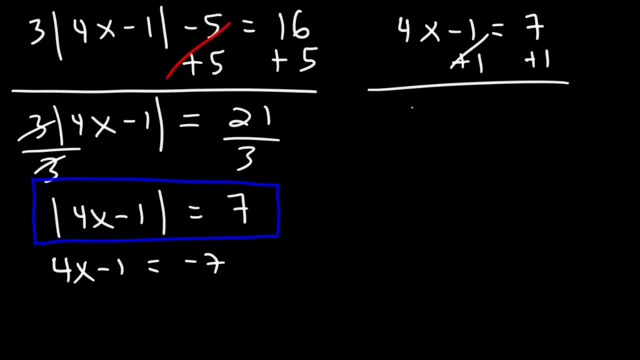 So for this one we'll add 1 to both sides. 7 plus 1 is 8.. And then we could divide both sides by 4.. And so 8 divided by 4 is 2.. So this is the first answer. 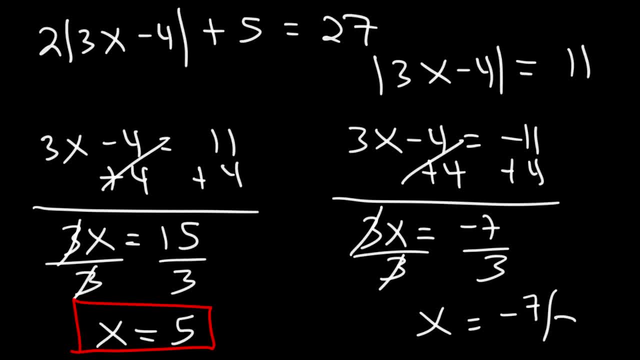 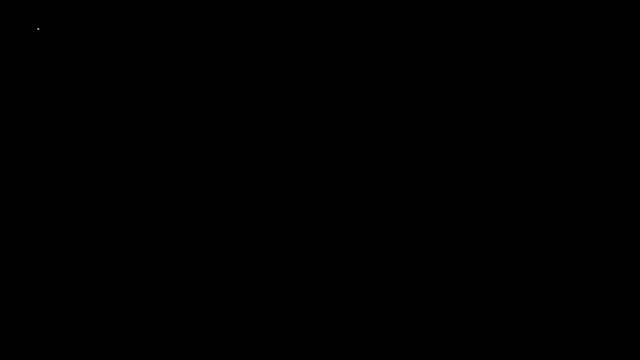 the second answer will be equal to a fraction, So it's going to be negative 7 over 3.. Okay, So these are the solutions to the original equation, And you could plug it in to see if it makes sense. if it works, Now let's go ahead and work on another example. So we're going to have 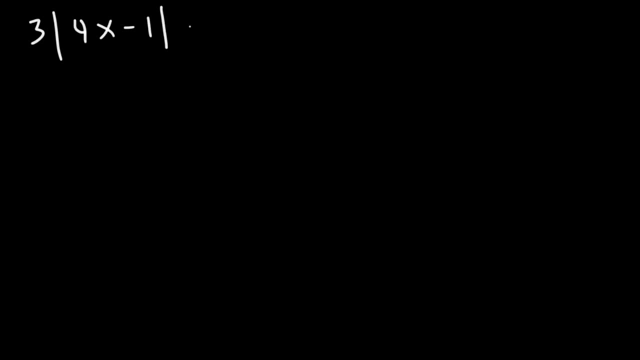 3 times the absolute value of 4x minus 1 minus 5, which is equal to 16.. So, for the sake of practice, pause the video and try that example. So we're going to begin by adding 5 to both sides of the equation. 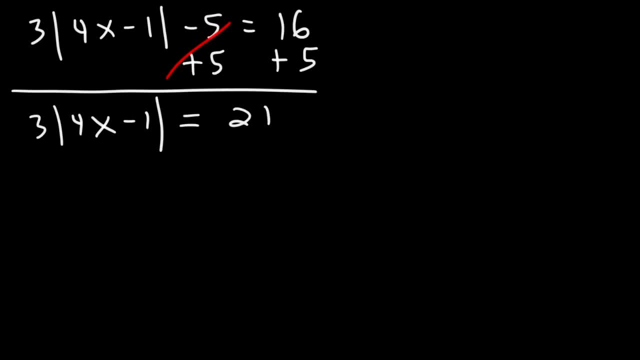 Now, 16 plus 5 is 21.. Next, let's divide both sides by 3.. And so 21 divided by 3 is 7.. Now, in this format, in this form, we can now divide both sides by 3.. And so 21 divided by 3 is 7.. 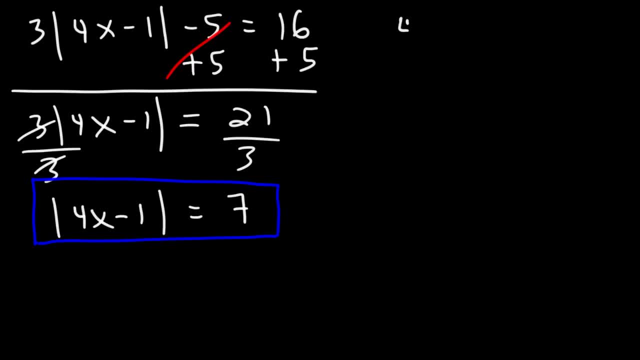 Now break it up into two equations. So the first one's going to be: 4x minus 1, is equal to 7. And the second one, 4x minus 1, is equal to negative 7. So for this one we'll add 1 to both sides. 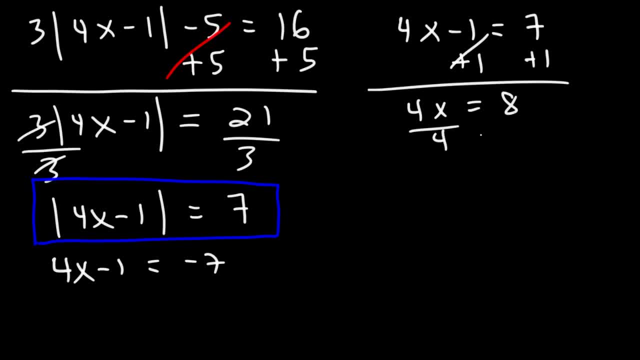 7 plus 1 is 8.. And then we could divide both sides by 4.. And so 8 divided by 4 is 2.. So this is the first answer: x is equal to 2.. For the next one, we're going to add 1 to both sides. 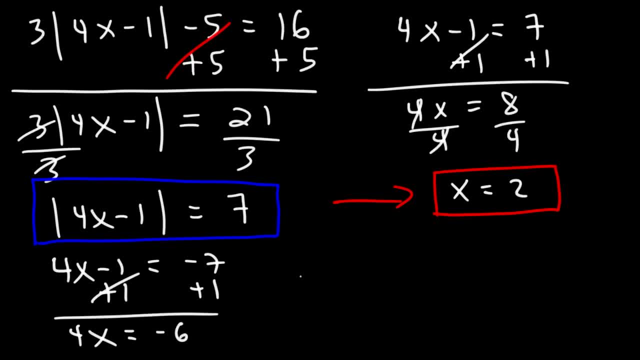 And negative 7 plus 1 is negative 6.. And then we're going to- let me do it over here, since I'm out of space- We're going to divide both sides by 4.. And so we get negative 6 over 4, which we can reduce that fraction if we divide the top number. 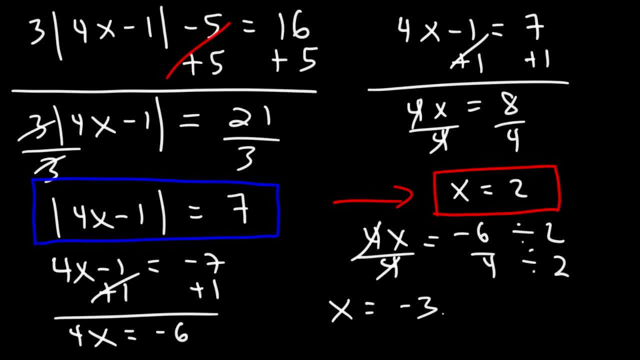 and the bottom number by 2.. Negative 6 divided by 2 is 3.. 4 divided by 2 is 2.. So the second answer is: x is equal to negative 3 over 2.. And so that's it for this problem. 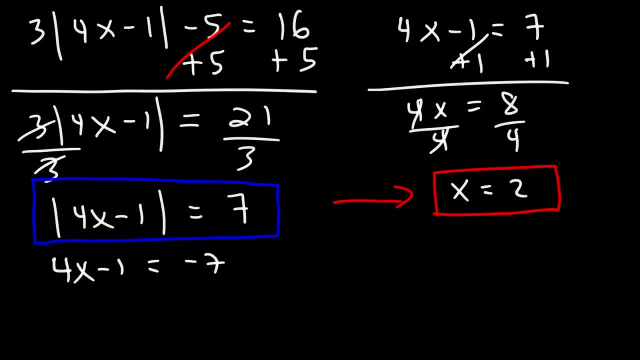 x is equal to 2.. For the next one, we're going to add 1 to both sides, And negative 7 plus 1 is negative 6.. And then we're going to- Let me do it over here, since I'm out of space- 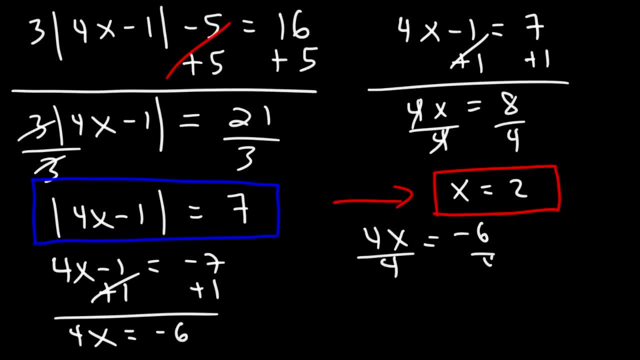 We're going to divide both sides by 4.. And so we get negative 6 over 4.. Which We can reduce that fraction If we divide the top number and the bottom number by 2.. Negative 6 divided by 2 is 3.. 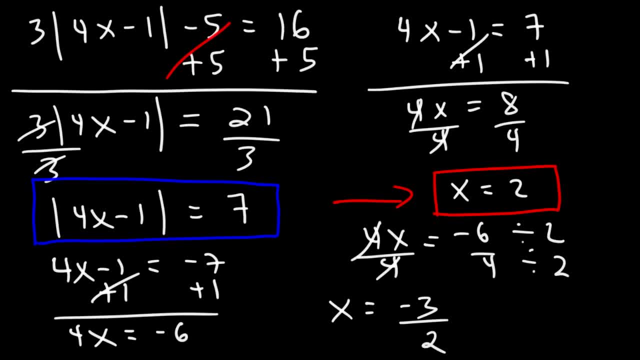 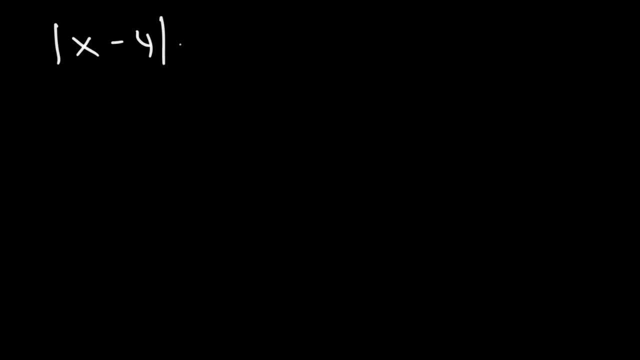 4 divided by 2 is 2.. So the second answer is: x is equal to negative 3 over 2.. And so that's it for this problem. Here's another one for you. The absolute value of x minus 4 plus 8 is equal to 3.. 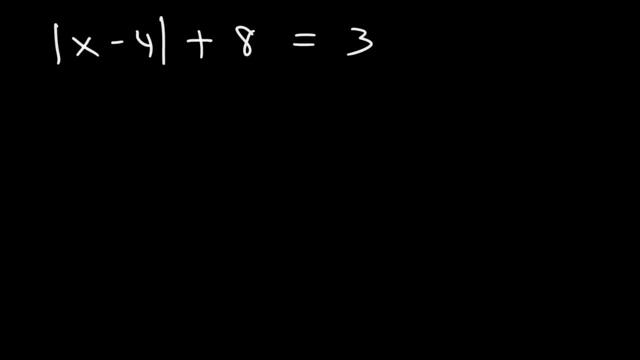 What is the answer? Well, the first thing we need to do in this problem is we need to subtract both sides by 8. And so we're going to have the absolute value of x minus 4 is equal to 3 minus 8,, which is negative 5.. 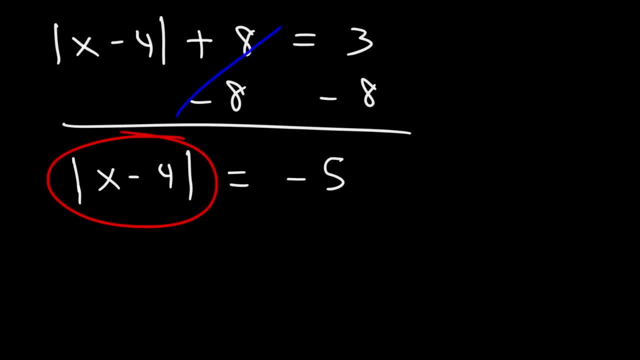 Notice the issue: The absolute value of something cannot equal a negative number, So therefore There's no solution for this problem. Here's another one: The absolute value of 7x plus 2 is equal to 4x plus 11.. 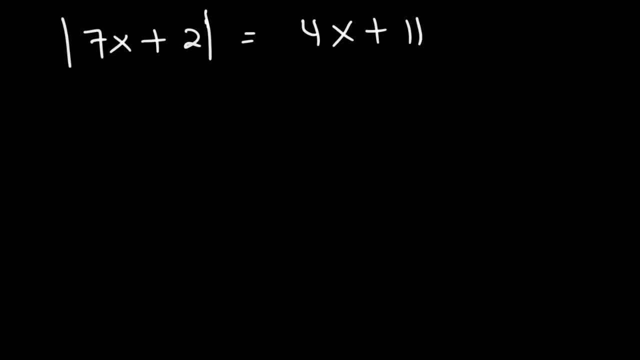 Go ahead and work on that one. So once again, we need to write two equations: The first one. The second one Will be exactly the same, But just without the absolute value. Now for the second one. all we need to do is multiply one of the two sides by negative 1.. 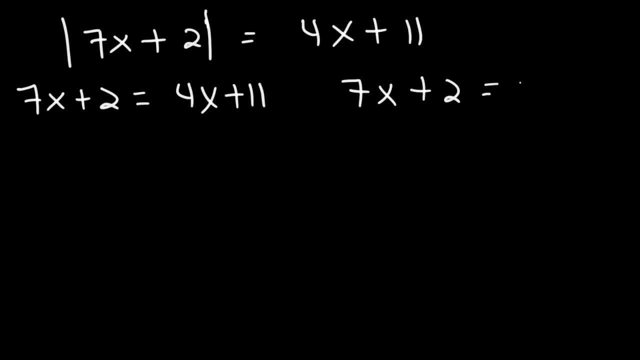 It really doesn't matter which one, So I'm just going to pick the right side. So I'm going to put a negative in front of 4x plus 11.. Now let's focus on the first one. Let's begin by subtracting both sides by 4.. 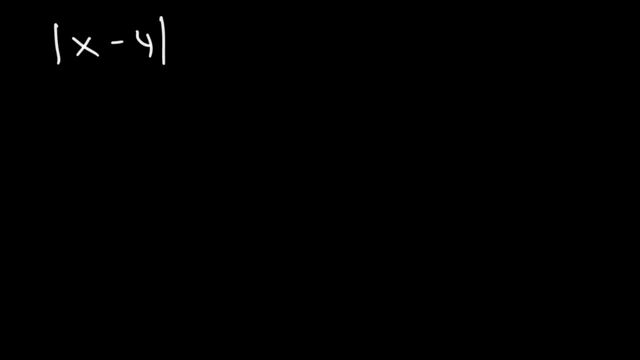 Here's another one for you. The absolute value of x minus 4 plus 8 is equal to 3.. What is the answer? Well, the first thing we need to do in this problem is we need to subtract both sides by 8.. 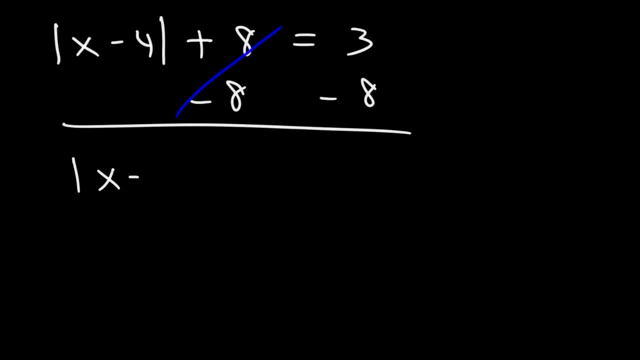 And so we're going to have: the absolute value of x minus 4 is equal to 3 minus 8, which is negative 5.. Notice the issue: The absolute value of something cannot equal a negative number. So therefore there's no solution for this problem. 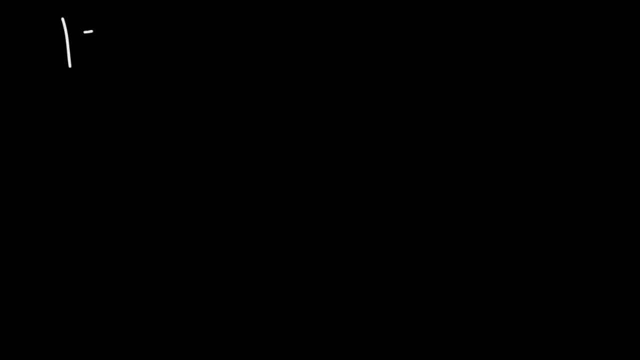 Notice that there's no solution for this problem. There's no solution for this problem. Here's another one. The absolute value of 7x plus 2 is equal to 4x plus 11.. Go ahead and work on that one. 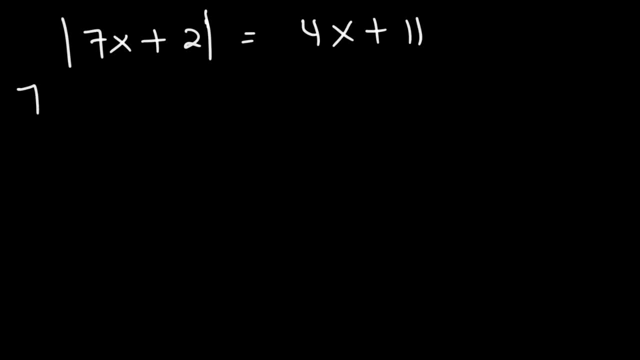 So once again, we need to write two equations. The first one will be exactly the same, It's just without the absolute value. Now for the second one one. All we need to do is multiply one of the two sides by negative one. It really doesn't matter. 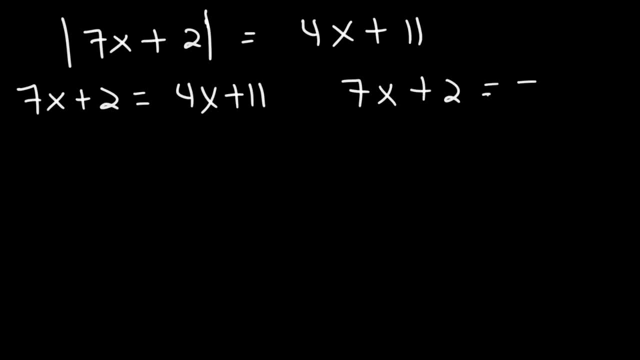 which one. so I'm just going to pick the right side. So I'm going to put a negative in front of 4x plus 11.. Now let's focus on the first one. Let's begin by subtracting both sides by 4,. 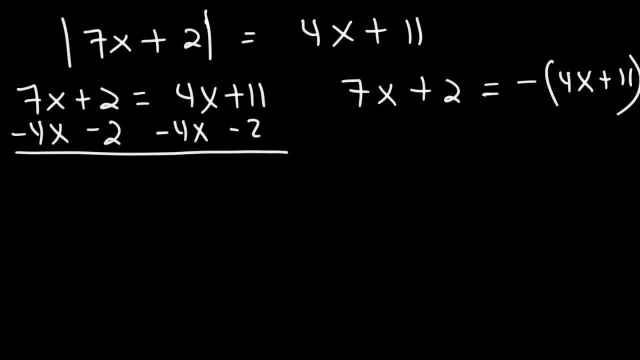 and at the same time let's subtract both sides by 2.. So the 2s and the 4s will cancel. I mean the 4x, 7x minus 4x is 3x, and 11 minus 2 is 9.. Now we'll need to divide by 3,. 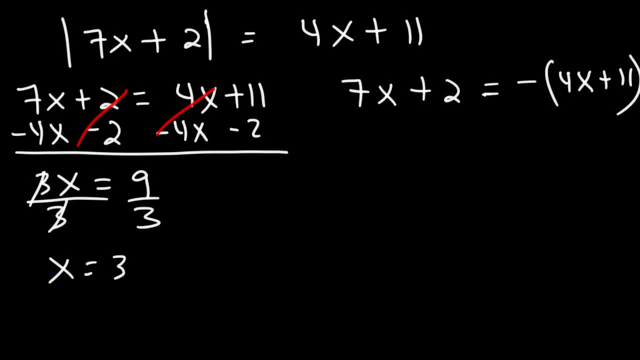 and so we get: x is equal to 3.. Now for the second problem. let's begin by distributing the negative sign first. So it's going to be negative 4x and negative 11. Now let's add 4x to both sides and at the same time let's subtract both sides by 2.. 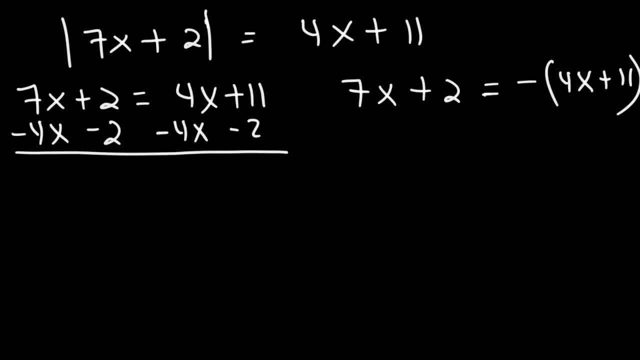 And at the same time let's subtract both sides by 2.. So the 2's and the 4's will cancel. I mean the 4x, 7x minus 4x is 3x, And 11 minus 2 is 9.. 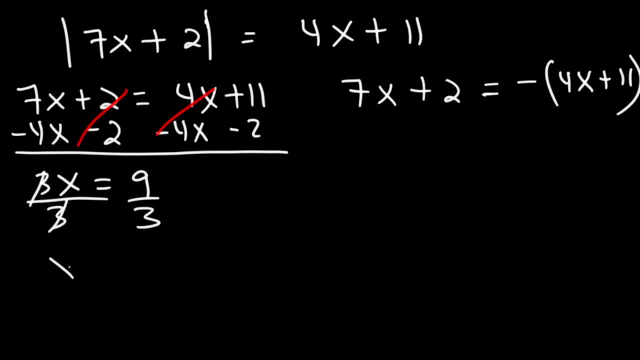 Now we'll need to divide by 3. And so we get: x is equal to 3.. Now for the second problem. let's begin by distributing the negative sign first. So it's going to be negative 4x. 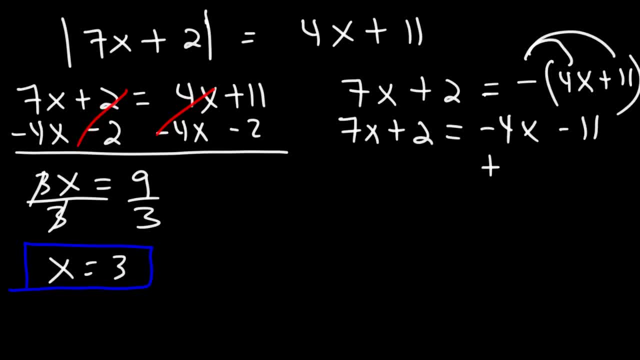 And negative 11. Now let's add 4x to both sides And at the same time let's subtract both sides by 2. So 2 and negative 2 will cancel, And negative 4x and 4x will cancel as well. 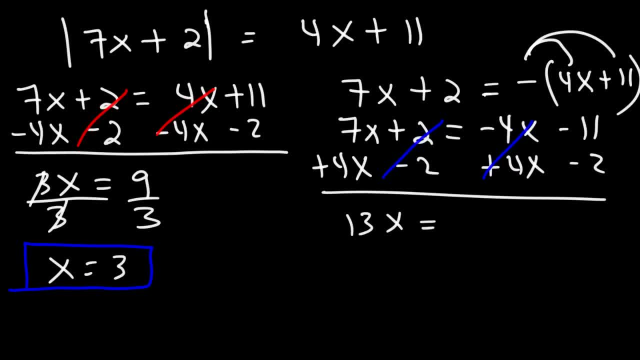 7x plus 4x is 13x- Negative. 11 minus 2 is negative 13.. Whoa, I did that wrong. 7x plus 4x is 11x, not 13x, But this is still negative 13.. 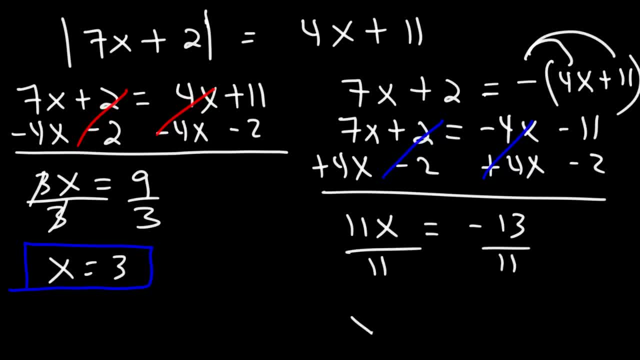 So if we divide both sides by 11, we're going to get x is equal to negative 13 over 11.. Now, for problems such as these, it's good to check to see if both answers work, if one of them works or if none of them works. 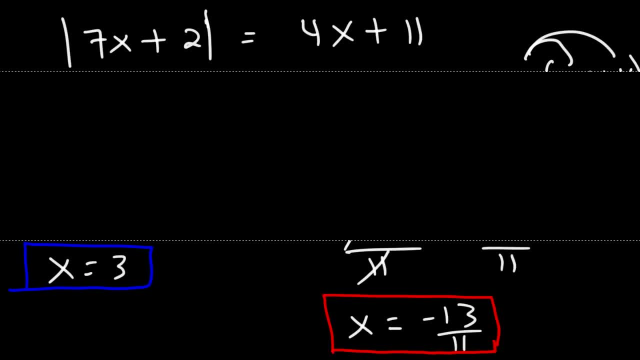 Let's start with: x is equal to 3.. Let me just clear away a few things. first, Replace an x with 3.. We're going to have this Now: 7 times 3 is 21.. And 4 times 3 is 12.. 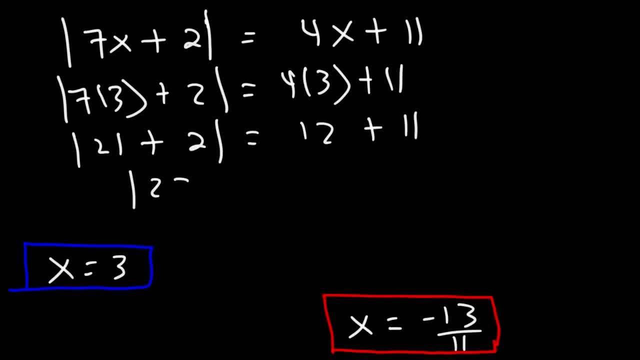 21 plus 2 is 23.. And 4 times 2 is 22.. And 4 times 3 is 21.. And 4 times 3 is 23.. And 11 plus 12 is 23.. 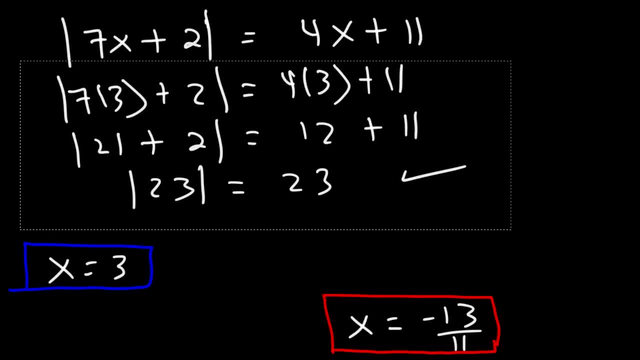 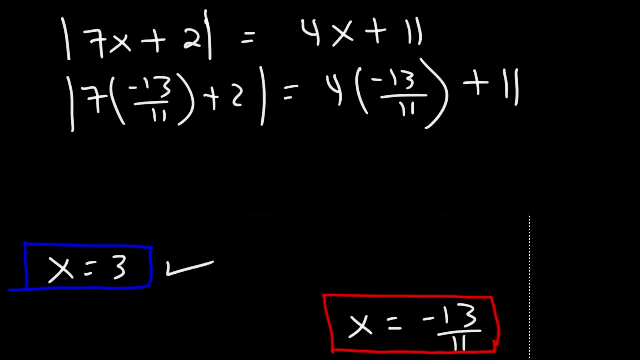 So this works. So this solution is correct. Now let's try the other one. So we have 7 times negative 13 over 11 plus 2.. I might need more space, so I'm going to get rid of this. Now, 7 times 13,, that's going to be 91.. 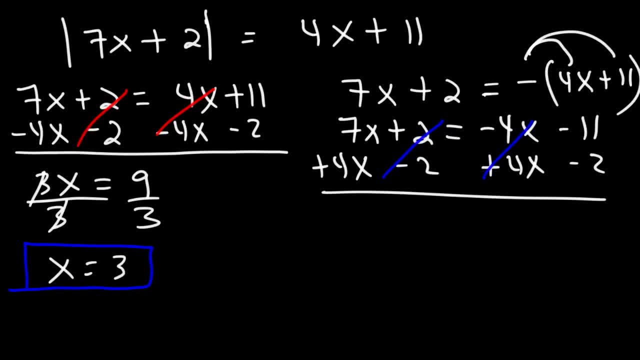 So 2 and negative 2 will cancel and negative 4x and 4x will cancel as well. 7x plus 4x is 13x, Negative. 11 minus 2 is negative 13.. Whoa, I did that wrong. 7x plus 4x is 11x, not 13x. 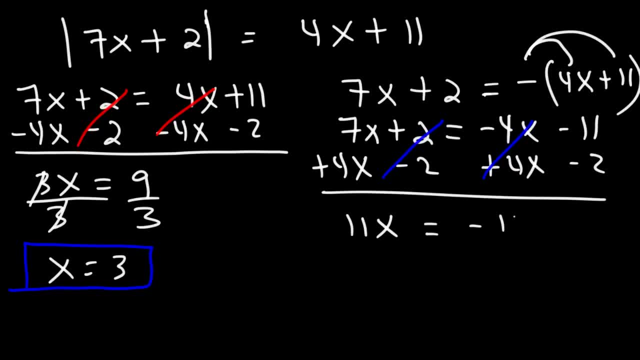 But this is still negative 13.. So if we divide both sides by 11, we're going to get: x is equal to negative 13 over 11.. Now, for problems such as these, it's good to check to see if both answers work, if one of them works or if none of them works. 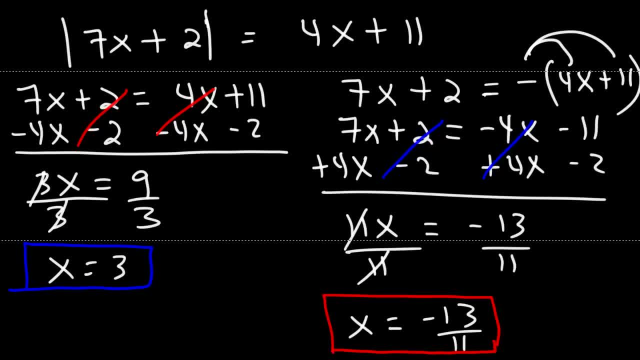 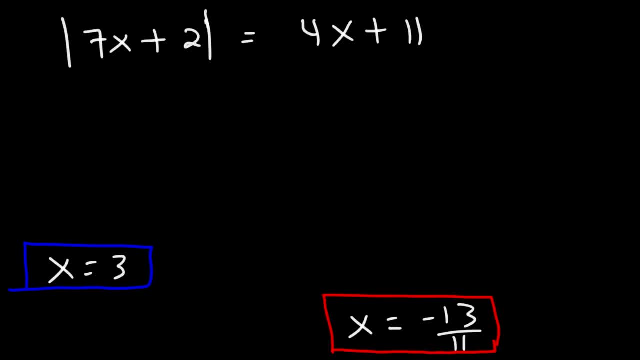 Let's start with: x is equal to 3.. Let me just clear away a few things. first, Replace an x with 3.. We're going to have this Now: 7 times 3 is 21,, and 4 times 3 is 12.. 21 plus 2 is 23,, and 11 plus 12 is 23.. So this works. 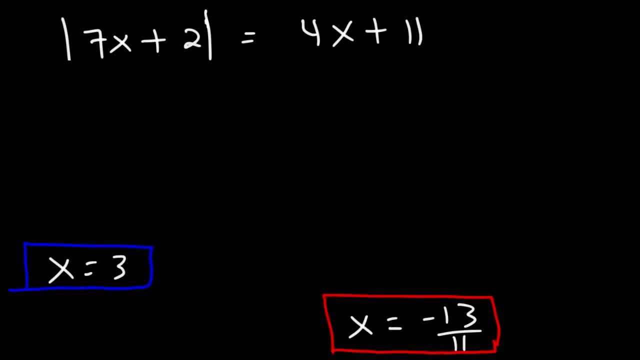 So this solution is correct. Now let's try the other one. So we have 7 times negative 13 over 11 plus 2.. I might need more space, so I'm going to get rid of this. Now, 7 times 13,, that's going to be 91.. 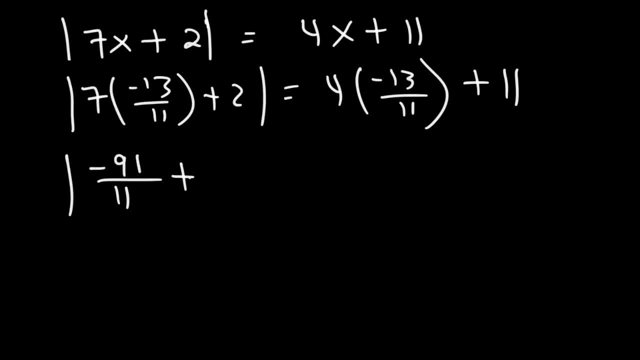 So I have negative 91 over 11.. Now 2, I'm going to change that. I need to get common denominators. So I'm going to multiply this by 11 over 11, and that's going to give me 22 over 11.. 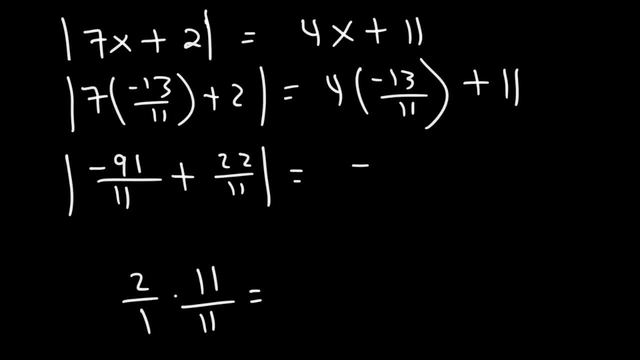 Now 4 times 13,. this is going to be negative 52.. Now this: I want to turn that into a fraction with common denominators. So I'm going to multiply this by 11 over 11.. And so that's going to be 121 over 11.. 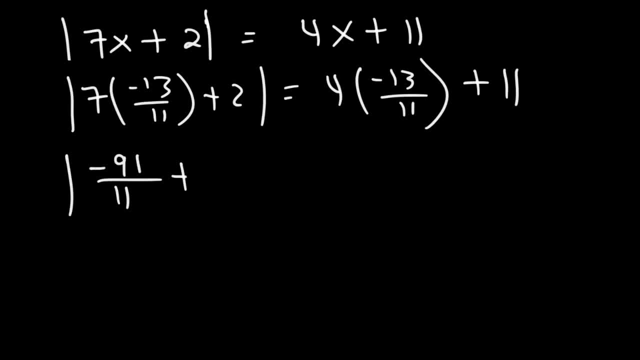 So I have negative 91 over 11.. Now 2, I'm going to change that. I need to get common denominators. So I'm going to multiply this by 11 over 11, and that's going to give me 22 over 11.. 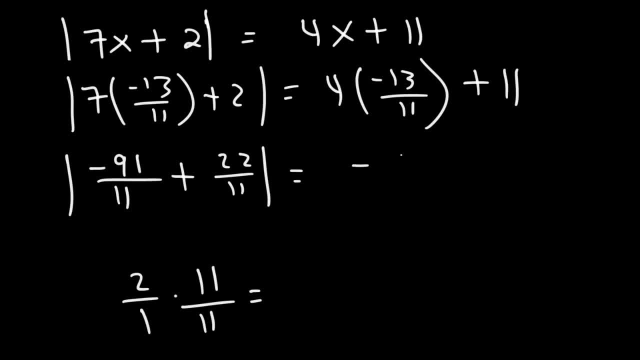 Now 4 times 13,. this is going to be negative 52.. Now this: I want to turn that into into a fraction with common denominators. So I'm going to multiply this by 11 over 11.. And so that's going to be 121 over 11.. 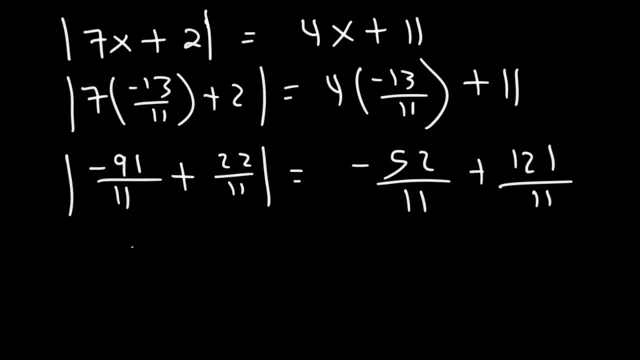 Negative 91 plus 22,. that's negative 69.. And negative 52 plus 121 is positive 69. The absolute value, The absolute value of negative 69 over 11 is positive 69 over 11.. So, because the left side is equal to the right side, 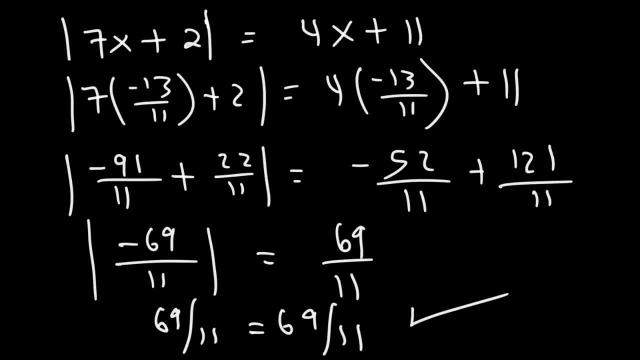 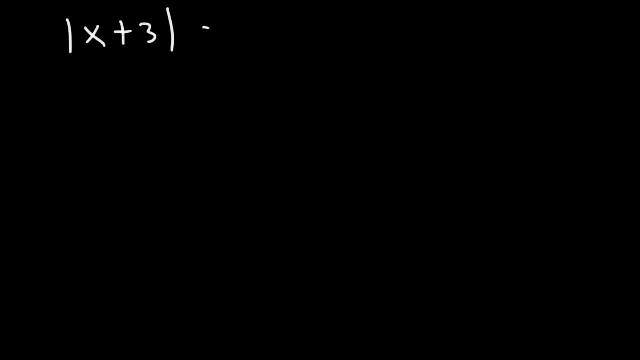 we could say that negative 13 over 11 is also another solution. Now what would you do if you have two absolute value expressions like this? Go ahead and try this problem. So the absolute value of x plus 3. is equal to the absolute value of x minus 11.. 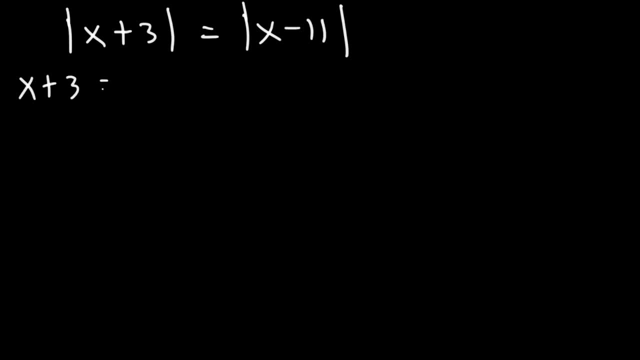 So, once again, we're going to write two equations. The first one is just going to be without the absolute value, And for the second one, all we need to do is multiply one of the two sides by negative 1.. And just to follow the same pattern, I'm going to multiply the right side by negative 1.. 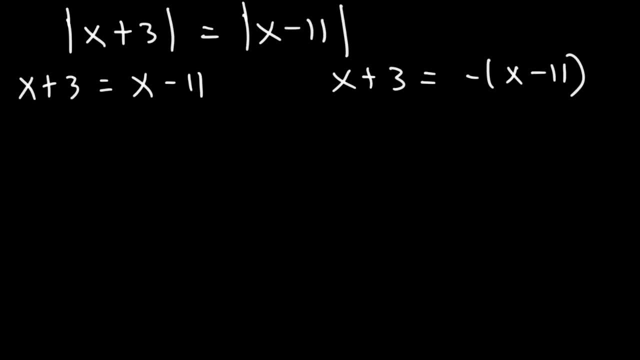 Now for the equation on the left side. if I subtract both sides by x, notice that they will both cancel, And so I'm going to have: 3 is equal to negative 11. And that makes no sense. That is not true. 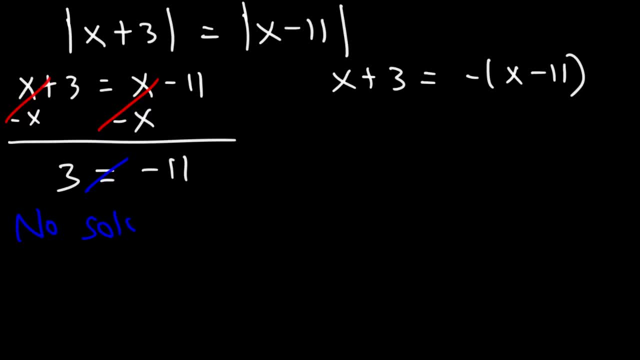 So there's no solution for this portion of the problem. Now for the next one. if we distribute the negative sign, we'll have negative x plus 11.. Now if we add x to both sides, we're still going to have an x variable on the left side. 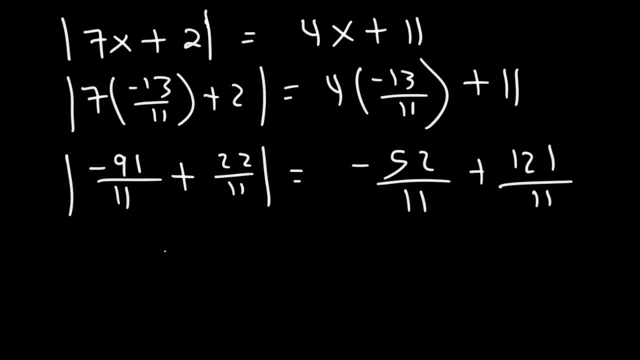 Negative 91 plus 22, that's negative 69. And negative 52 plus 121 is positive 69. The absolute value of negative 69 over 11 is positive 69 over 11.. So because the left side is equal to the right side, we could say that negative 13 over 11 is also another solution. 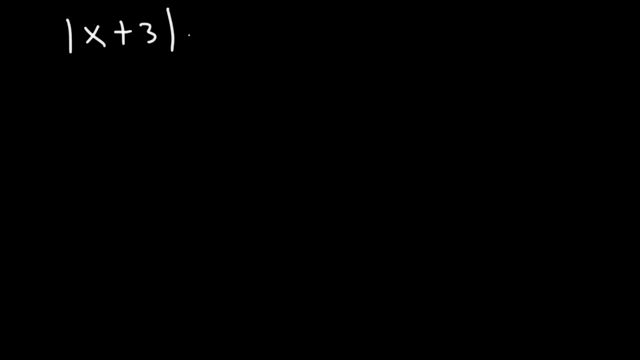 Now what would you do if you have two absolute value expressions like this? Go ahead and try this problem. So the absolute value of x plus 3 is equal to the absolute value of x minus 11.. So what's the answer? Once again, we're going to write two equations. 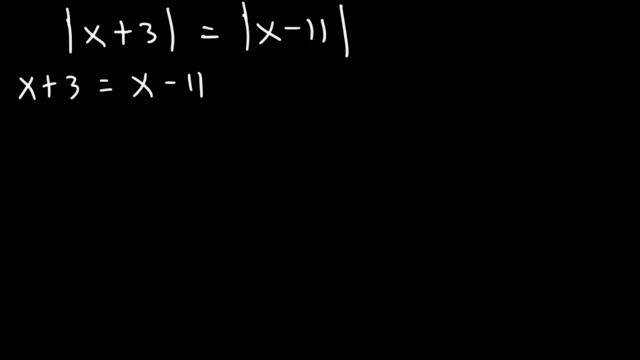 The first one is just going to be without the absolute value, And for the second one, all we need to do is multiply one of the two sides by negative 1.. And just to follow the same pattern, I'm going to multiply the right side by negative 1.. 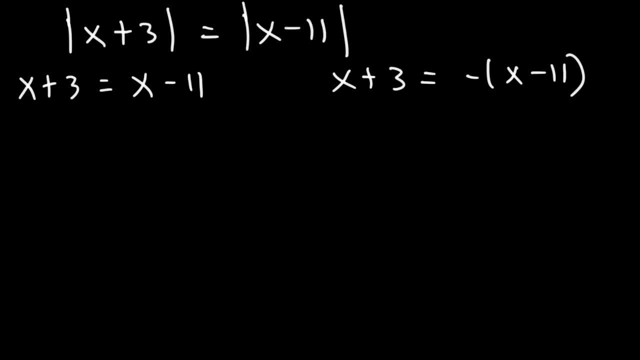 Now for the equation on the left side. if I subtract both sides by x, notice that they will both cancel, And so I'm going to have: 3 is equal to negative 11. And that makes no sense. That is not true. 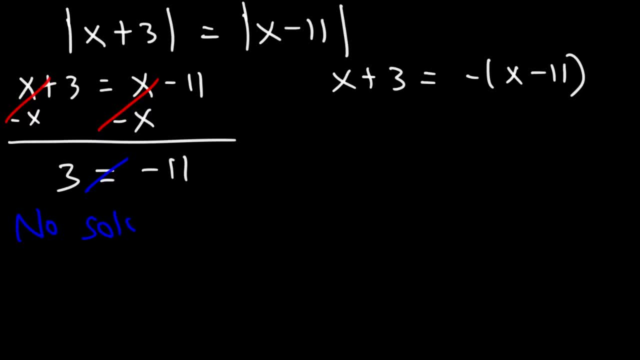 So there's no solution for this portion of the problem. Now for the next one. if we distribute the negative side, we'll have negative x plus 11.. Now if we add x to both sides, we're still going to have negative 11.. 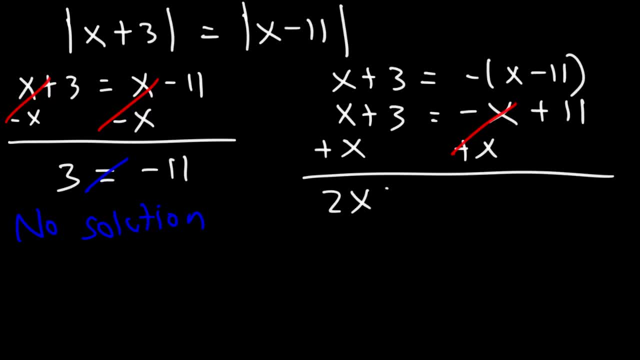 So we're going to have an x variable on the left side. x plus x is 2x. Now let's subtract both sides by 3.. So 11 minus 3 is 8. And then we'll divide both sides by 2.. 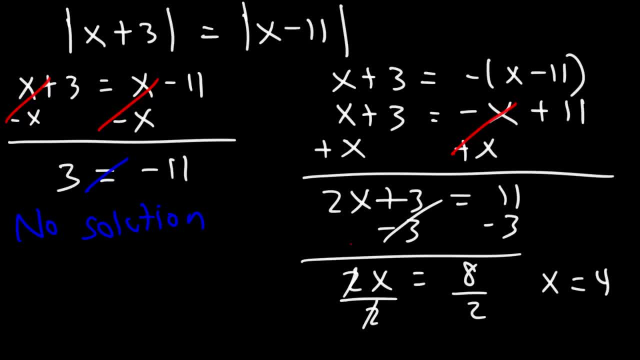 So 8 divided by 2 is 4.. So we have one potential answer: x is equal to 4.. But just to make sure, let's go ahead and check it. So this is going to be 4.. So this is going to be 4.. 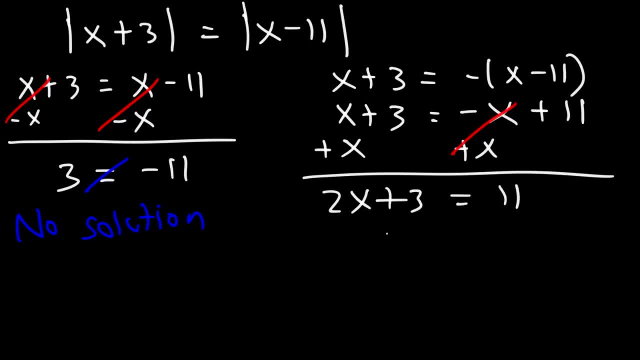 x plus x is 2x. Now let's subtract both sides by 3.. So 11 minus 3 is 8.. And then we'll divide both sides by 2. So 8 divided by 2 is 4.. 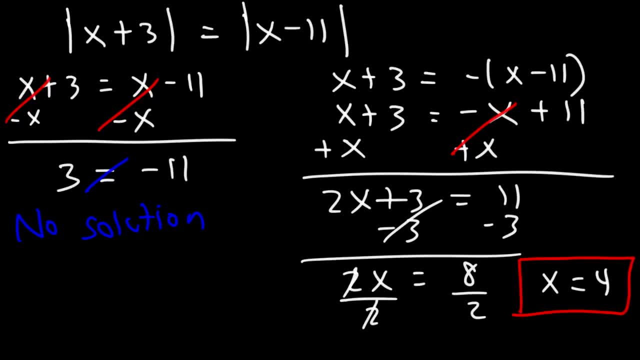 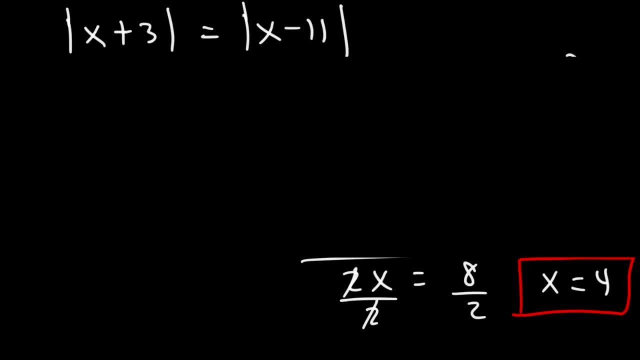 So we have one potential answer: x is equal to 4.. But just to make sure, let's go ahead and check it. So this is going to be 4 plus 3. And here we're going to have 4 minus 11.. 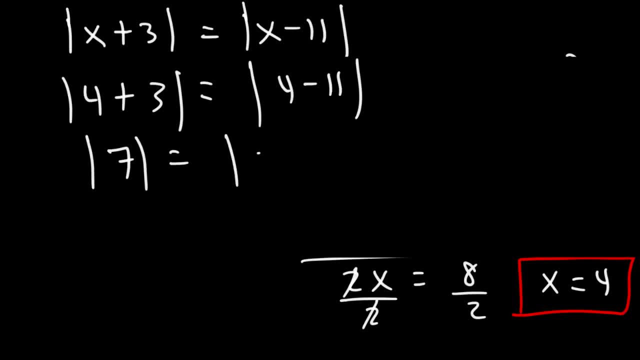 4 plus 3 is 7.. 4 minus 11 is negative, 7.. The absolute value of 7 is 7.. The absolute value of negative 7 is also 7.. So these two are equal to each other, which means this is the correct answer. 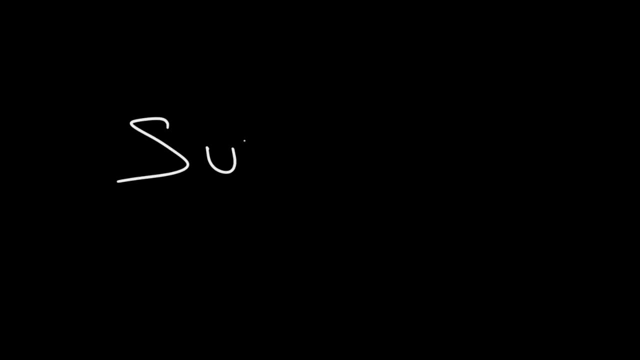 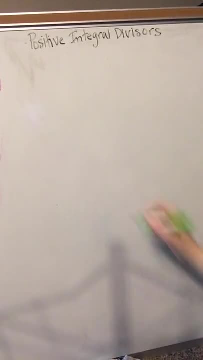 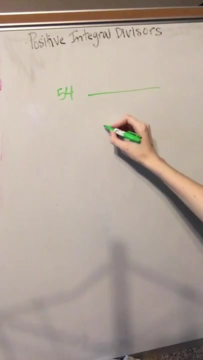 Now we're going to do positive integral divisors. So the question may ask you: for example, how many positive integral divisors does 54 have? So what you can do is you can imagine a little 54 and you can make yourself a little imaginary table in. 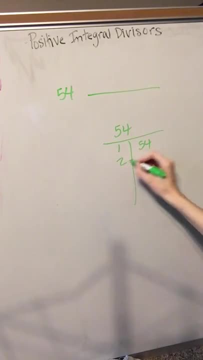 your head You can go 1 times 54,, 2 times 27,, 3 times 18, and 6 times 9.. So you go: oh, there's 8.. But a better way is to do this trick. So what you do is divide 54 in your head into its prime numbers. You. 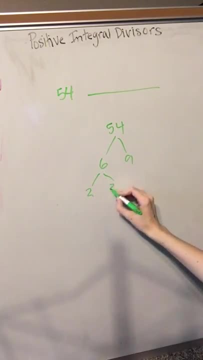 have 6 times 9,. those aren't prime numbers. so you do 2 times 3, and 3 times 3.. All prime numbers. So every time a prime number shows up, you add 1.. So there's 1,, 2,, 3,, 4 prime numbers. Do 4 times 2, and you get 8 as your answer.